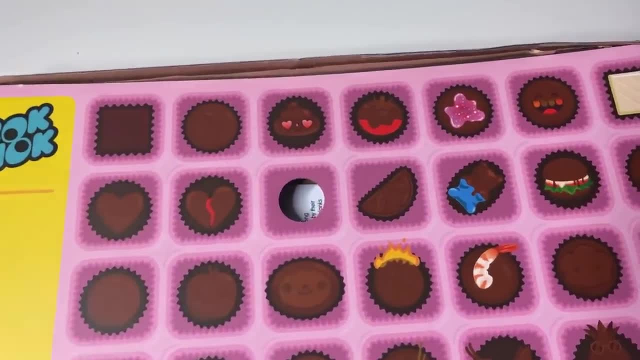 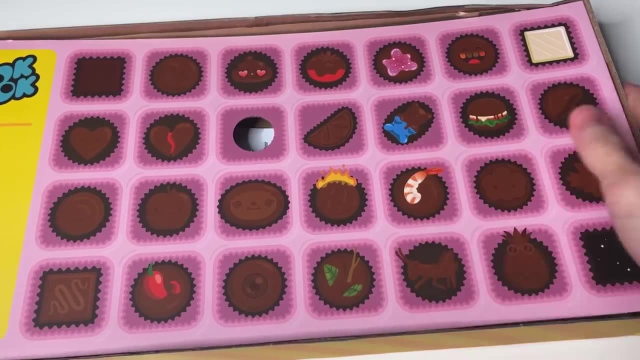 Whoa, look at this. Alright, so it's like a bunch of chocolates and stuff like in a row. Look at these. These look so great. What do you think? my favorite one is Probably the Gummy Bear one. Look at that one. It looks so good. It's got like blue on it. Whoa, these all look so cool. Broken Heart. 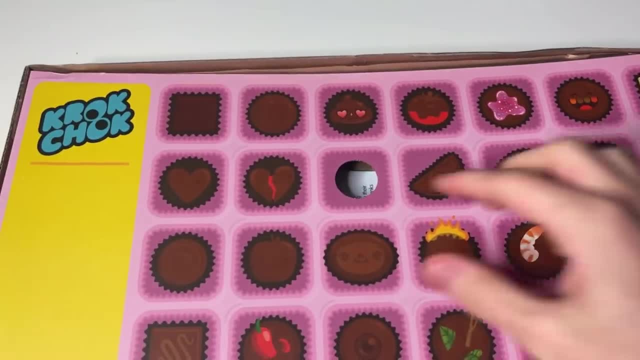 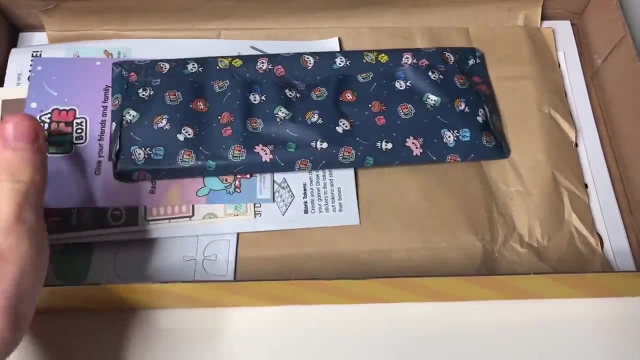 and there's a pineapple- Whoa, look at the Galaxy one That looks pretty awesome. Alright, let's just open this. Let's open this up right here and oh, already, some cool, exciting goodies inside. I am so excited for this, Oh my gosh. Okay, Wow, There is a lot of stuff in here. Look at the sloths. Oh my gosh. 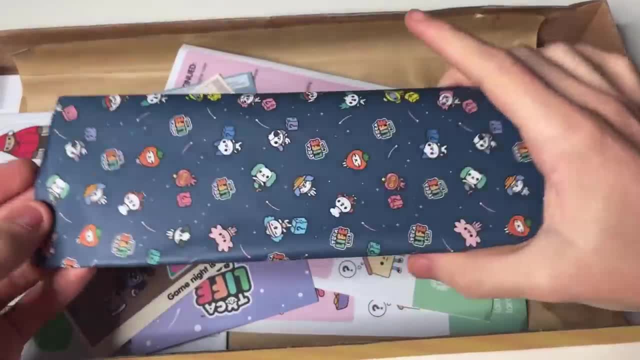 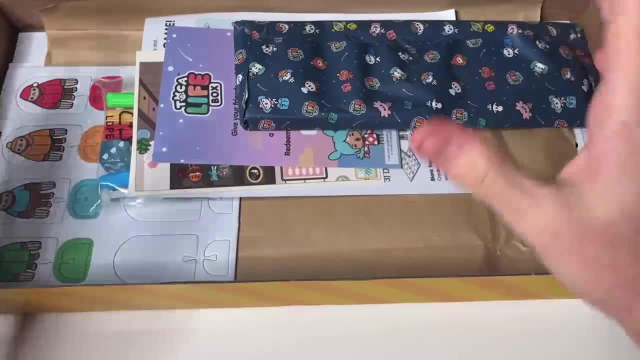 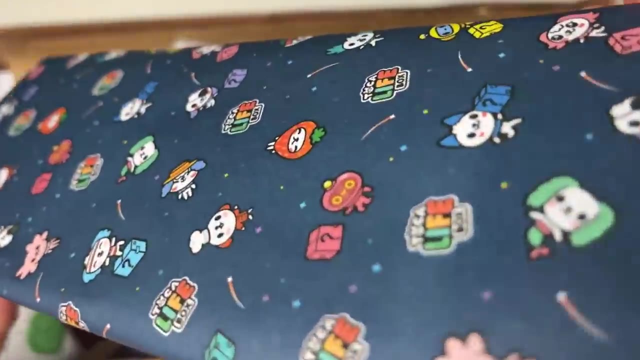 this is so cool. Okay, Right, So today we're going to let's just first- Alright, let's just first- open this kind of package right here, with all the crumpets on. Oh my gosh, This wrapping paper is so cute. 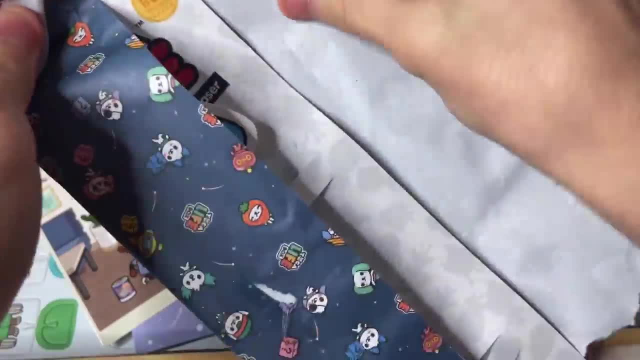 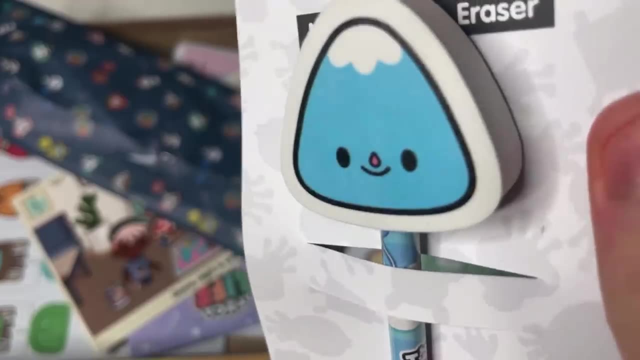 So cute. Alright, let's open it up, This cute little present. Let's see what's inside. What is this? Is this Whoa? look at this. It's a Nora pencil and eraser. Oh, it's a box exclusive This. 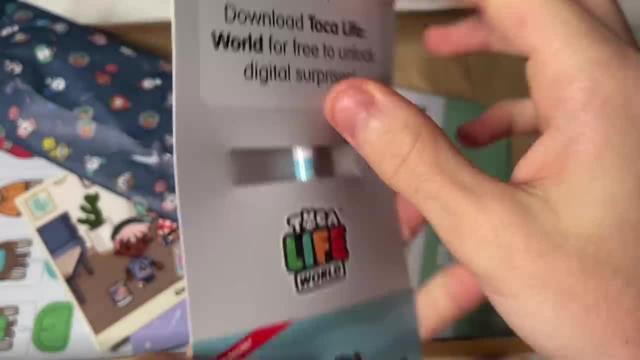 is so cool. It's got Toga Life on it. Whoa, it's got a balloon- the pattern. Oh, there's the download code to download Toga Life World. You should definitely get it. It's an amazing game And. 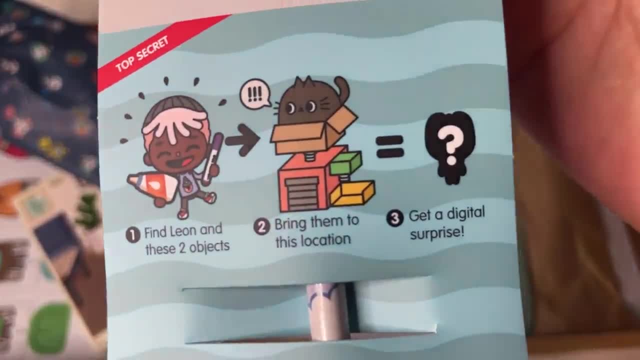 there's- oh, there's- the top secret crumpet, which I did make a video on a while ago. Some of you guys already found this out. So, yeah, that's pretty cool. Look at that. That's awesome. So nice, I love. 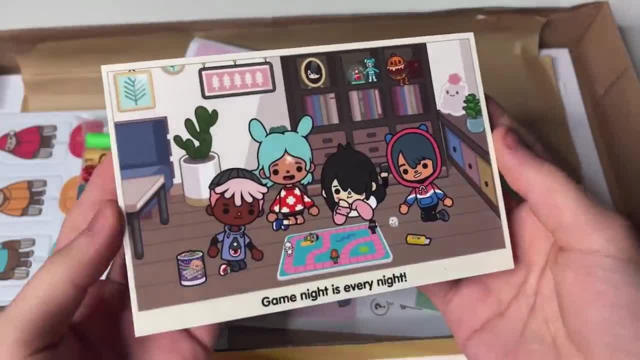 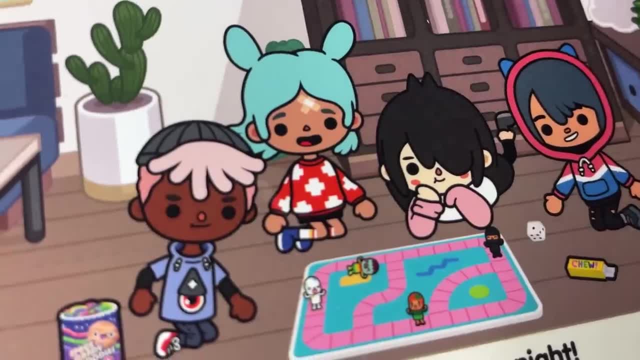 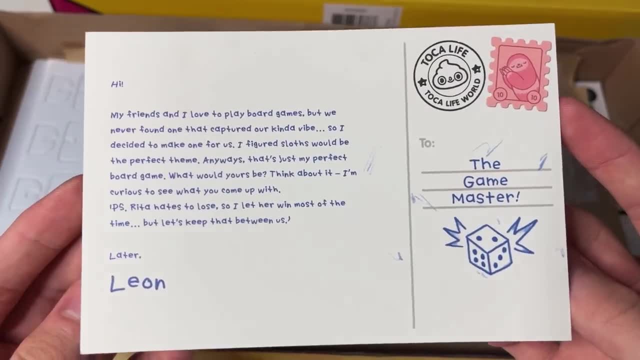 It looks like the whole gang right here- Rita, Leon, Nari Zeke- They're all chilling playing a board game. That is pretty cool And it says on the back here: hi, my friends and I love to play. 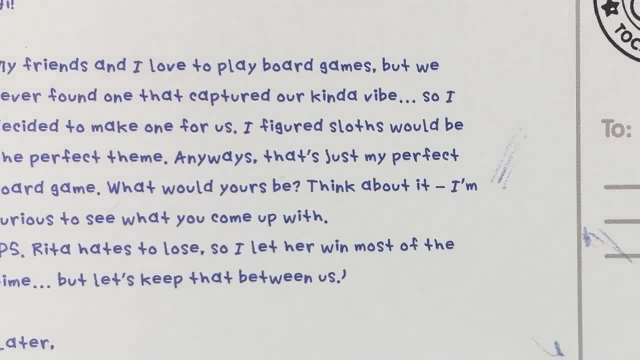 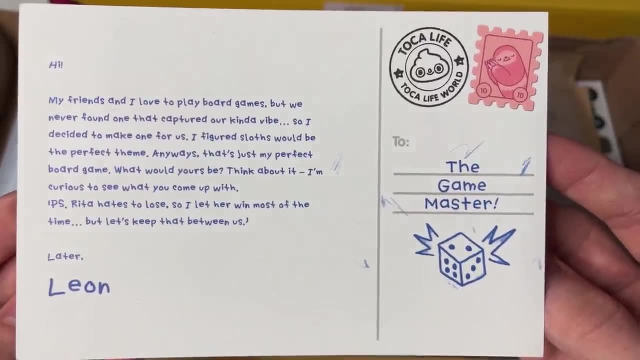 board games, but we never found one that captured our kind of vibe, So I decided to make one for us. I figured sloths would be the perfect theme. Anyways, that's just my perfect board game. What would yours be? Think about it. I'm just curious to see what you'd come up with PS. 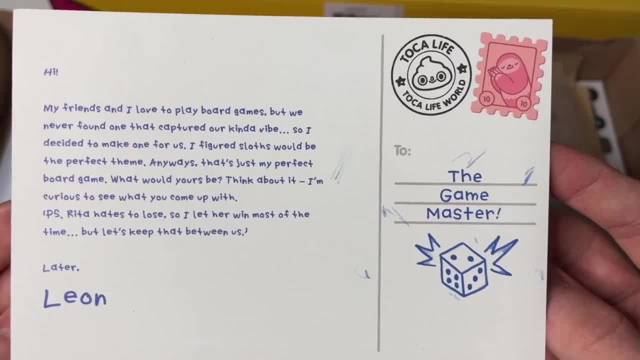 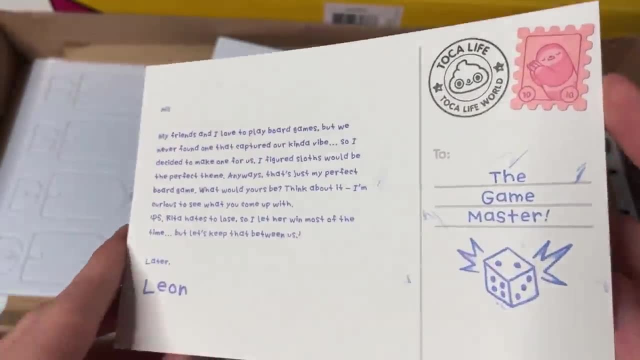 Rita hates to lose, so I'd let her win most of the time. But let's keep that between us Later, Leon. So it's like Leon wrote that and it's to the Game Masters, which I think is pretty much us. 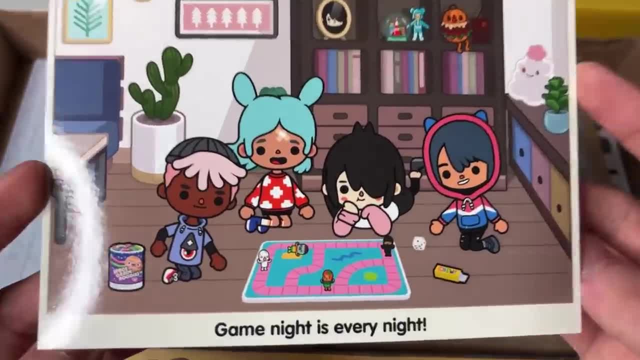 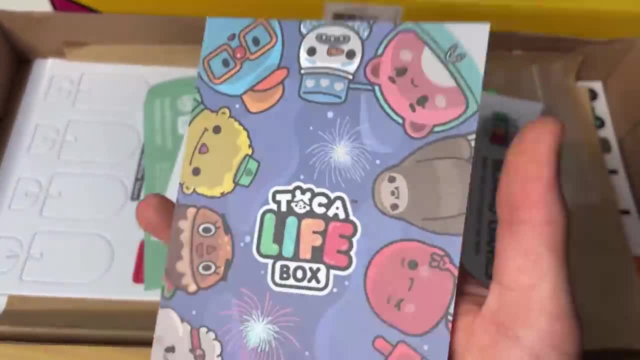 And that is so cool. Honestly, these kind of postcards kind of represent what's in the box, So like this is like the board game. It kind of feels like we have to maybe create our own and play one. So that's pretty cool. We also have another 15% off discount code. These things are 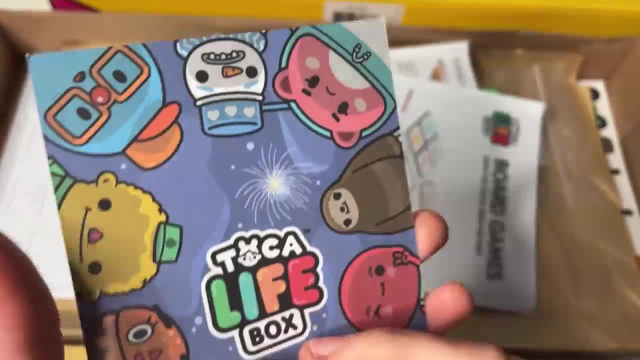 amazing. Honestly, I love the art for them. They're so cute. I love like all the characters around it. I see that all the time. It's so cute, I love that. But let's see this. Oh, okay, We have. 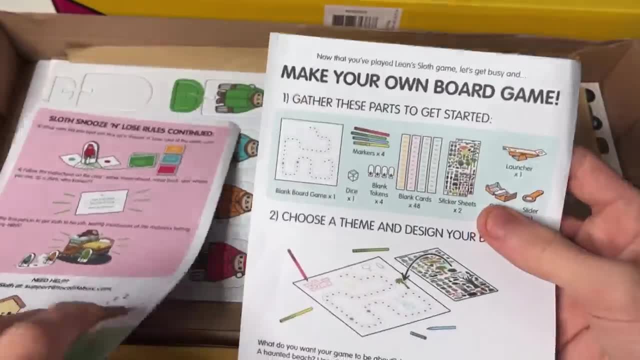 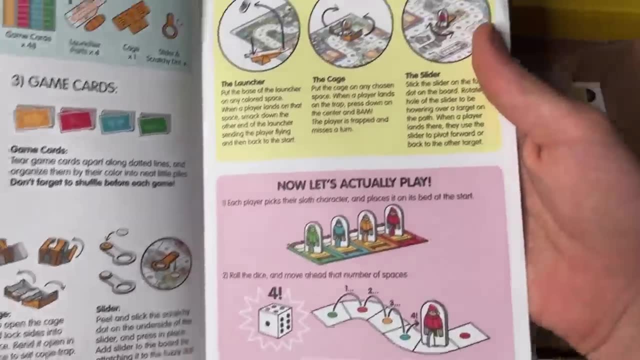 yes, Is this? make your own board game? Oh my gosh, This is so cool. Look at this board games. Oh, wow, I think these are the instructions for it. That's so cool. Look at this. Oh my gosh, I'm so. 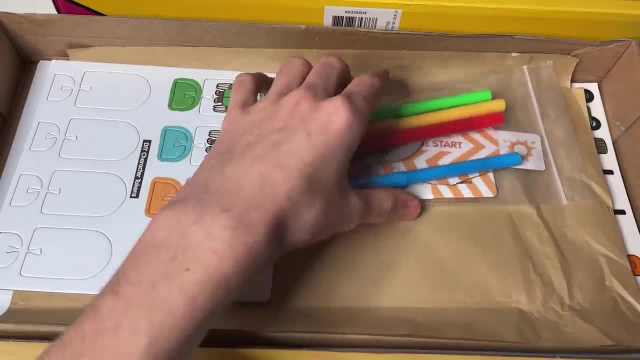 excited. I can't wait to get straight into this. Okay, We're just going to move them aside for now. But oh my gosh, look at this. These like the got pencils and stuff traps in there. That is so cool. 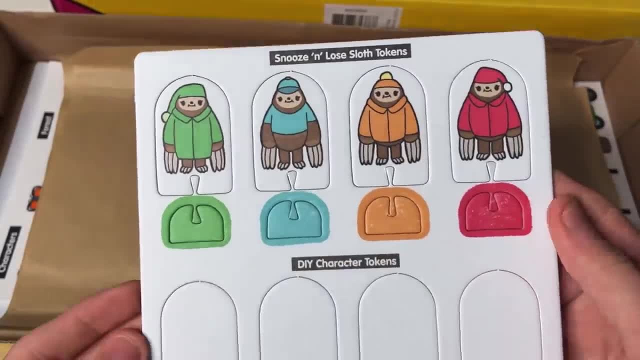 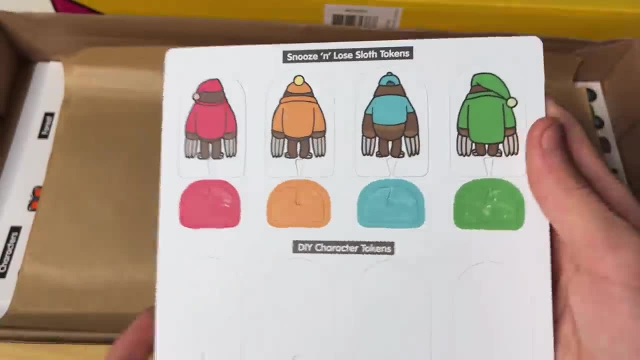 And we got sloths, of course, as well. All these- I think these are the characters For the board games- and- oh look, DIY character tokens. It looks like we get to create our own as well, Of course. that is going to be so fun. Wow, Look at that. All right, Let's see what else is in. 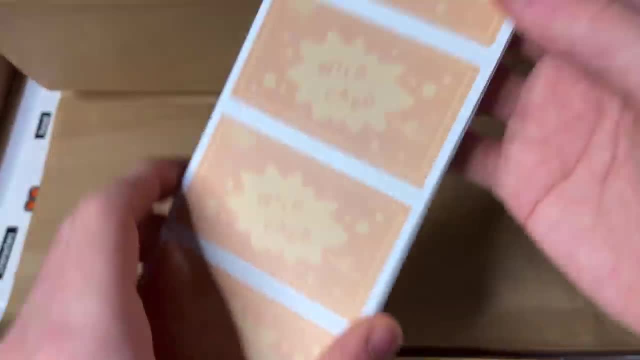 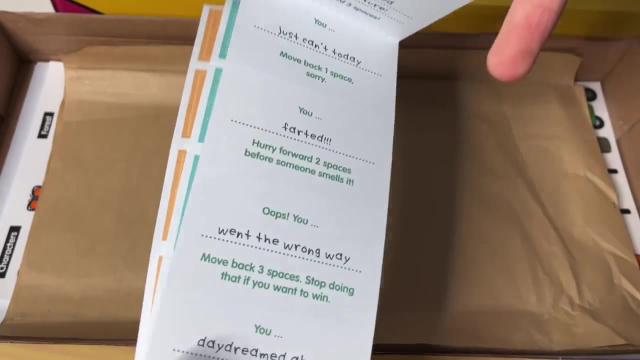 the box right here We got: Oh, what are these cards? Yeah, looks like they're cards. Wild cards, Okay, Except challenge and stuff. What are these These? Oh, okay, So let's see. Oops, you went the. 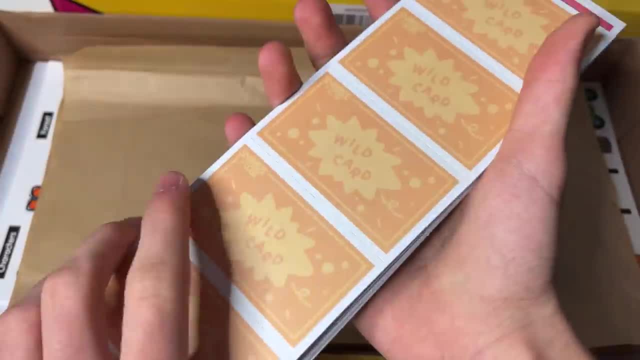 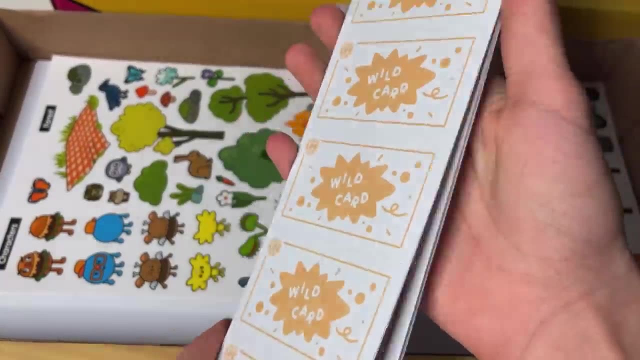 wrong way. Move back through spaces. Stop doing that if you want to win. That's pretty cool. So these are like the cards for when you pick out in the board game. Let's see, Oh, we got more cards. I think these look like maybe the other board game for when you create your own. Let's see, Yeah, 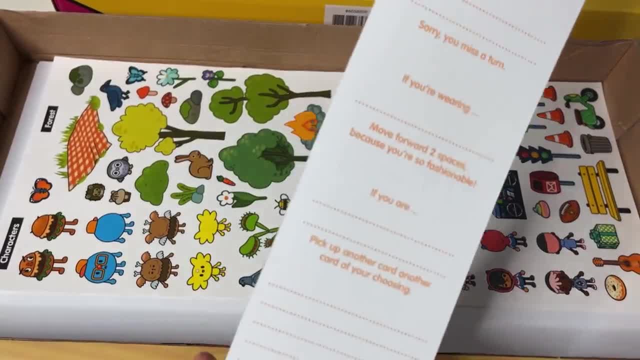 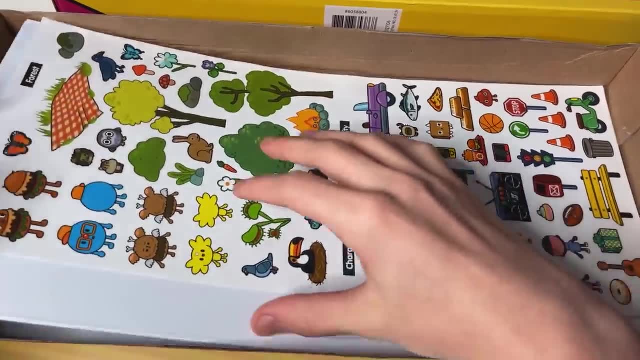 they are. Look see. Oh whoa, that's so cool, We get to write our own. That's awesome, That's so cool. All right, let's put them aside. Oh, stickers, I absolutely love stickers. Look at this Wow. 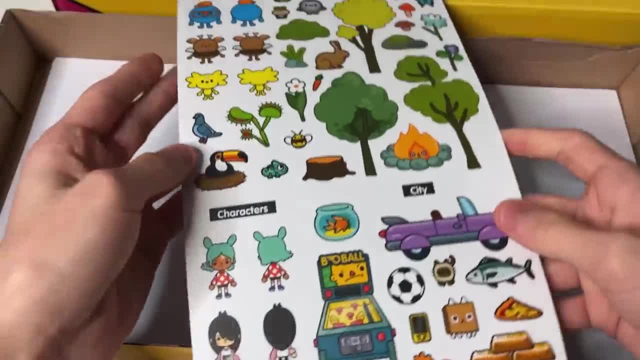 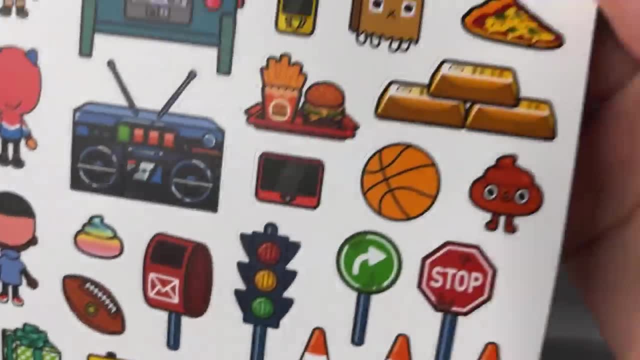 there are so many. Okay, let's get these out. Look at this. They're like different sections and stuff. Oh whoa, characters in the forest And you have like the gang and all the city. Look at all the cool items and stuff. That is so cool. 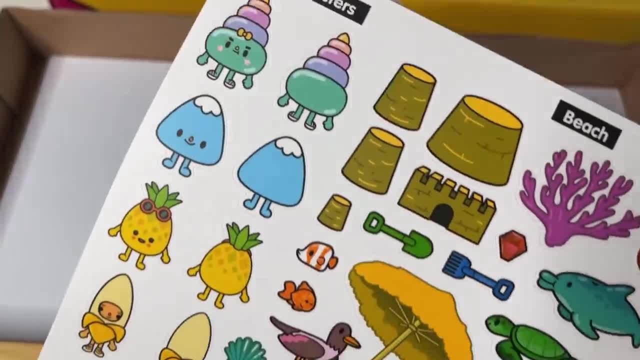 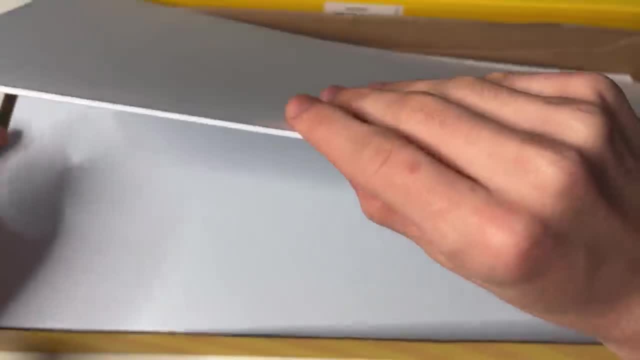 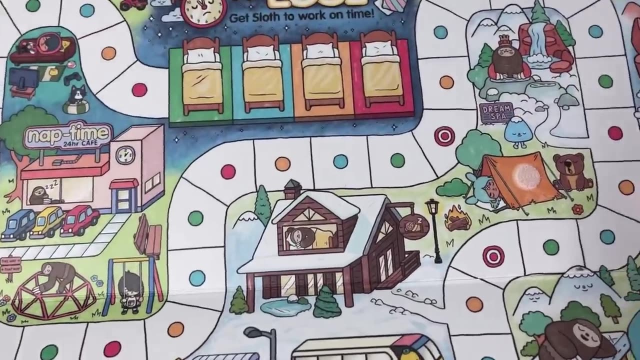 Look at that. And we've also got beach, beach theme. Whoa, oh, there's a shark there and a haunted house. He's like the locations and so like world. That's awesome. And what are this? Is this like a? these are board games. Whoa, that is. Whoa, look at this. This is so cool. Whoa, that is. 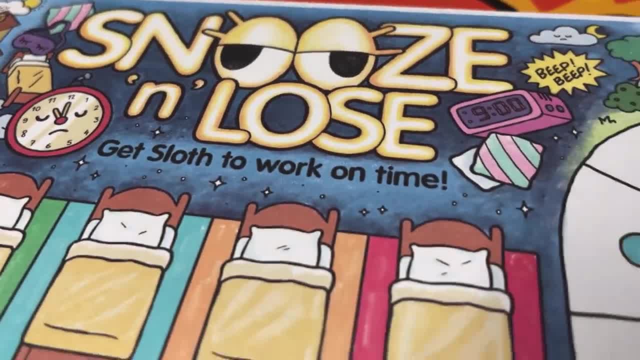 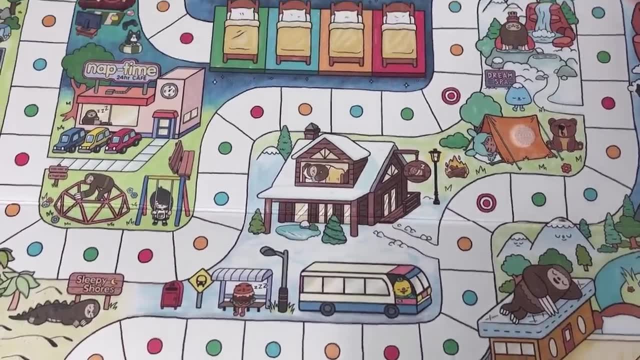 awesome. Look at the detail. This is like the snooze and lose. get sloths to work on time. That's awesome. So get to have like the sloths in the bed They got to traverse their way through the. get to like their workplace, which is this thing, Like the factory. they get to sleep. Look at this. 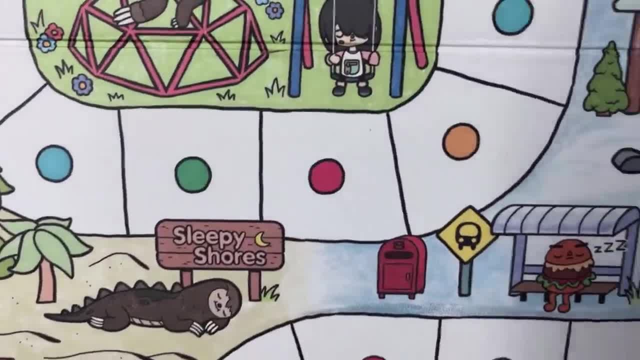 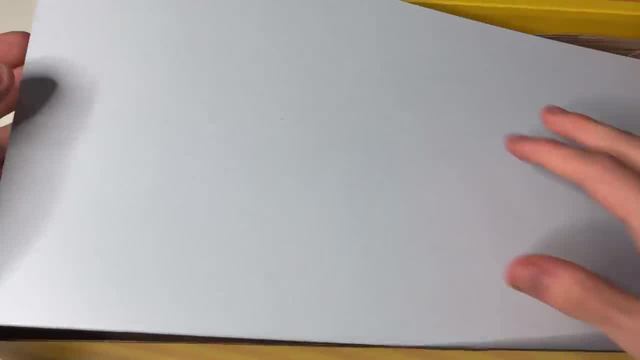 slumber park: Whoa, look at all of this. sleepy shores. There's the winter cabin with the little guy sleeping in there. Look at all of this. It's like all different locations, It's like world. That's awesome. We also got another board right here. Yes, this is where we get to create our own. 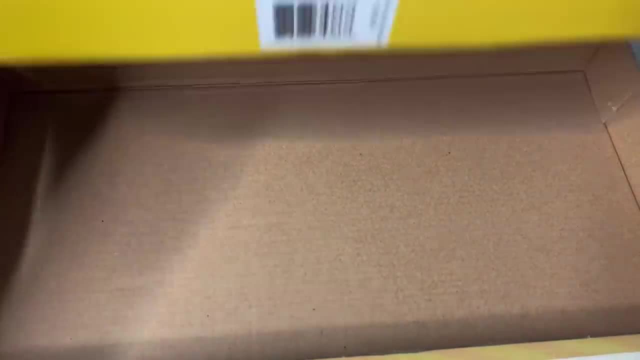 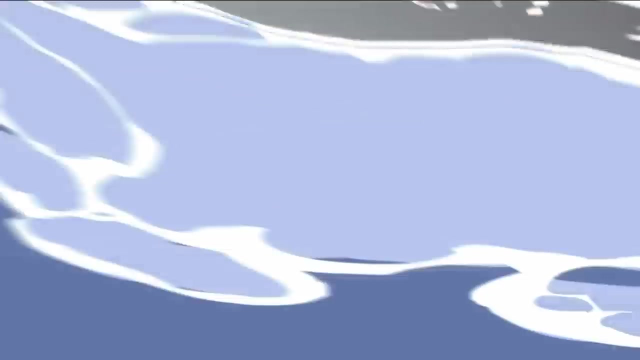 as well. That is awesome. Okay, I'm gonna move them aside. We're gonna close the box. That's pretty much everything in it. That is so cool. Let's set things up and see what we're gonna do. Let's do this, All right. so here we are. We're back. Let's see. Okay, so we got the instructions. 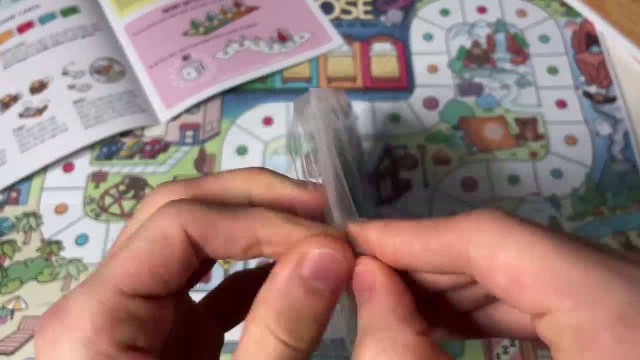 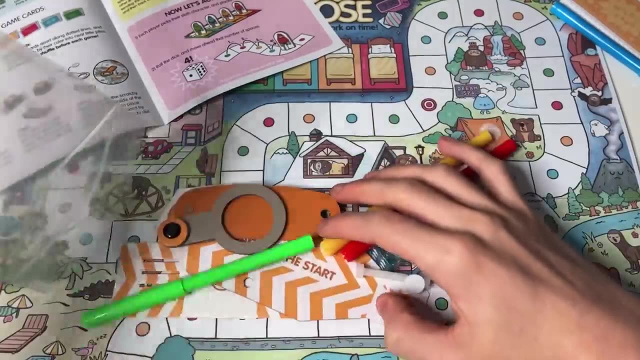 right here And we got like this bag, So let's open it up right here And like, let's see all the goodies inside. I can't believe there's like pens and a bunch of stuff in here. Look at this screws died like a dice. Okay, let's open this up, Let's see. Okay, so we got this thing right here. 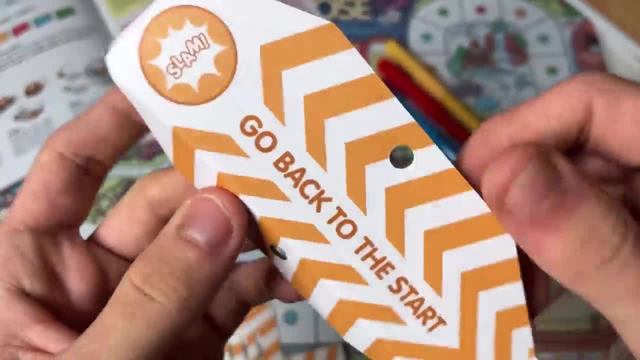 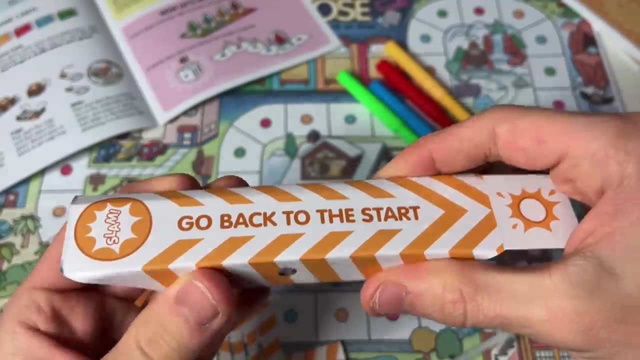 which I think is like the. it says it's like a catapult, So we got to fold the sides right here like this And then fold that over like that. So these are like different traps. What That is cool, Like like traps on a board game. Okay, this is very cool. I'm so interested. 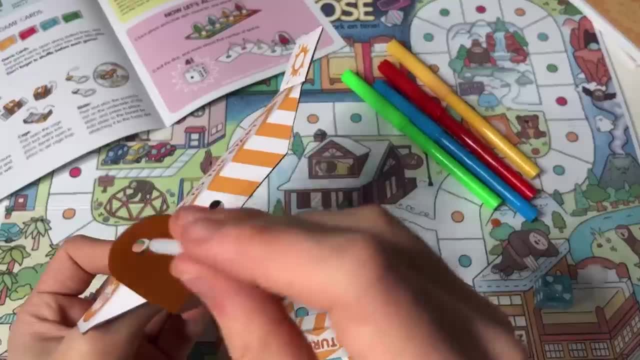 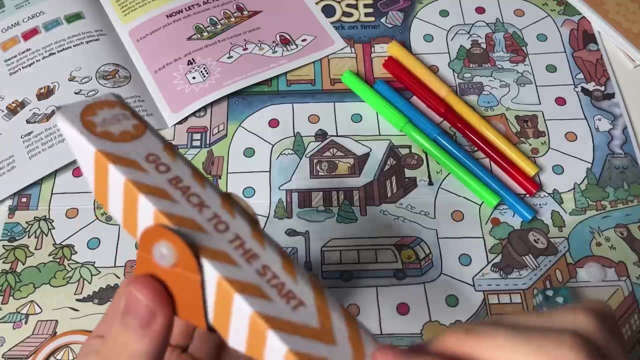 to see what this is all about. So we got to fold this over, put this in here and we need to get a screw. put the screw in that hole like. this is kind of like similar to the basketball one in my other unboxing video. It's kind of like the basketball, so you put your character on the end. 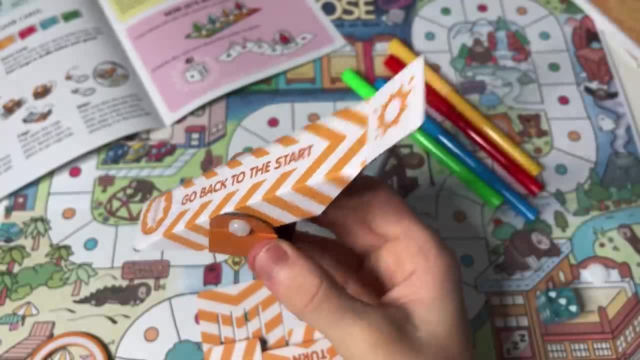 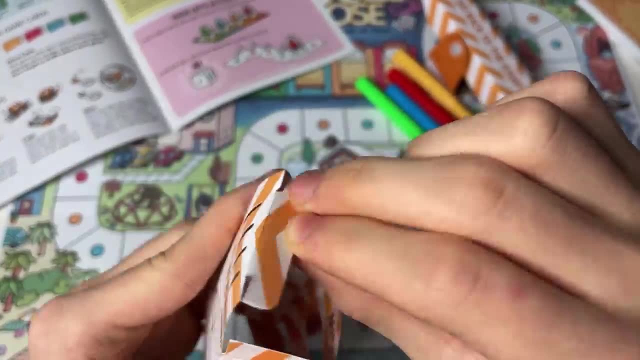 like this, and then you slam this down like that, Boom, And it says: go back to the start. I do not want to land on that trap. That would be awful. We got this trap right here, I think I just got to make it into a box, I think. So let's just do that real quick and then fold this bit like here: 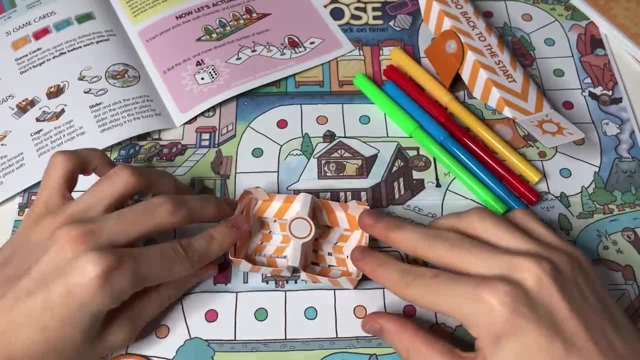 Okay, so I folded it all up and it's kind of like I need to open it up like this kind of like a bear trap or, like you know, a sloth trap which is so cool. So say, you get your character just walking. 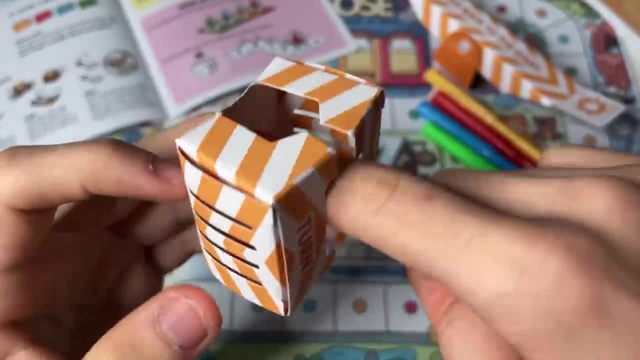 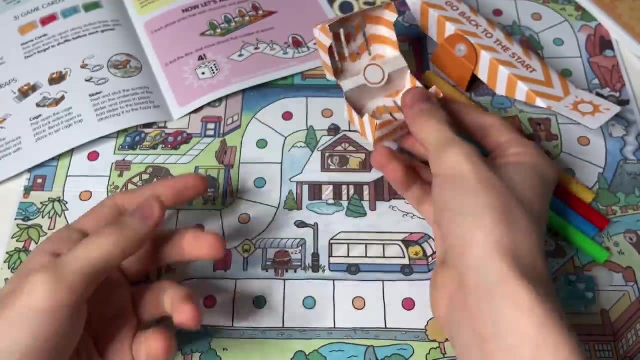 along like this. He steps on this bit like that and boom, my fingers trapped, It's so, it's so cool And so like, once you're in that you basically trapped and you miss a turn. That's awesome, That is so cool, I love that. And then we also have this kind of like: 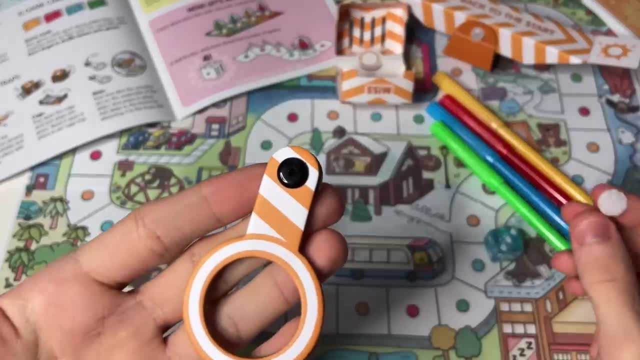 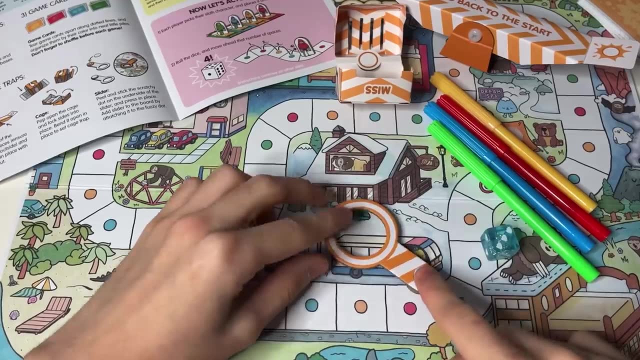 spinny, rotating thing. So it's like when you traverse through like the stages and that you can skip different sections, So you put the Velcro thing on here and then you basically just place it on the board and like move. like that I think, Yes, I think you just like basically put it on. 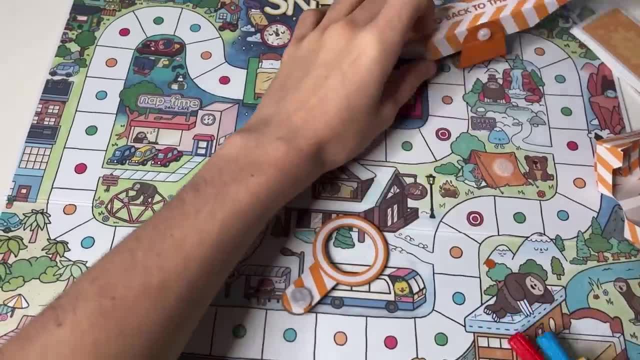 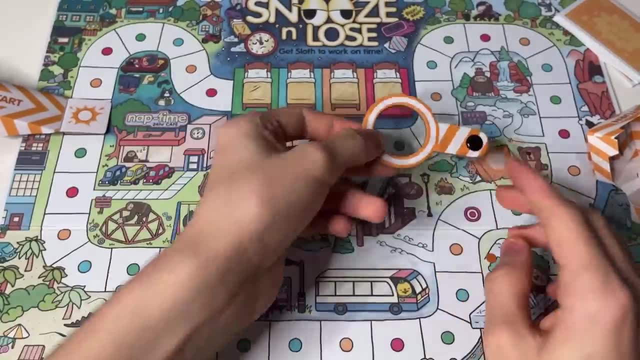 a spot and then you get to move around. That's pretty cool. And then we also have just some other like drawing things for your own board game. But I think I'm going to put the catapult right here, like that, And then I'm going to put this- I'm going to Velcro it onto this bit, like here: 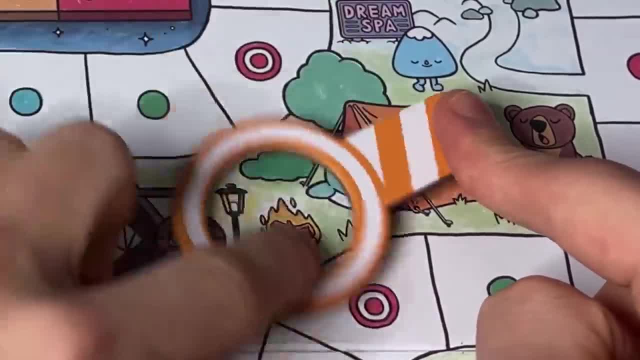 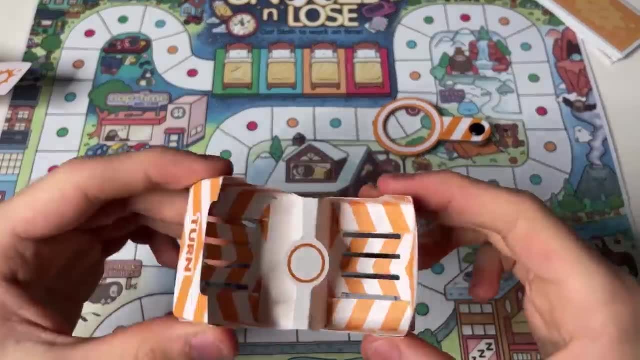 and then put them on the two. I only just realized. so I need to put them like that. See, they're different, So put, the Velcro is just attached to like that, which is very nice, And then I have a bear trap which I think I'm. 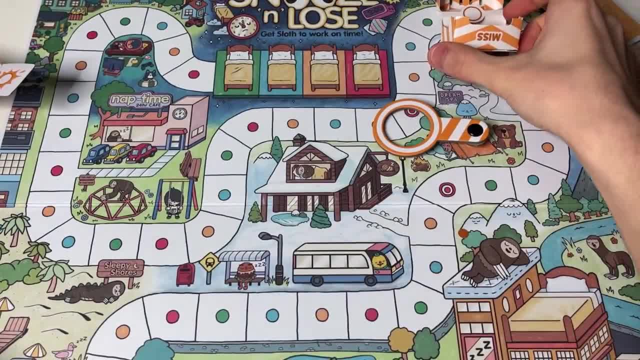 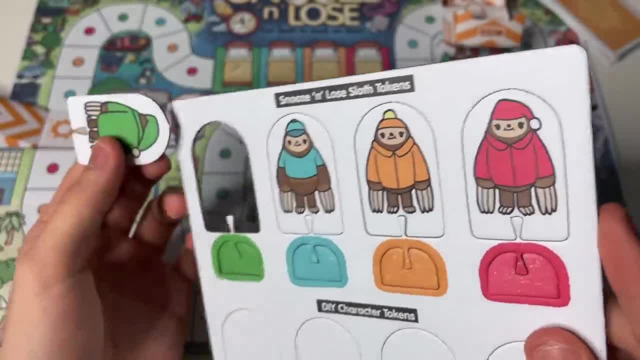 going to put right there, right there, right at the top- Awesome, That is so nice, And we've also got our characters as well. I'm going to take out the green soft for now. Green is honestly a very nice color, So we're going to get the stand right here. It's pretty easy. All you need to do is put. 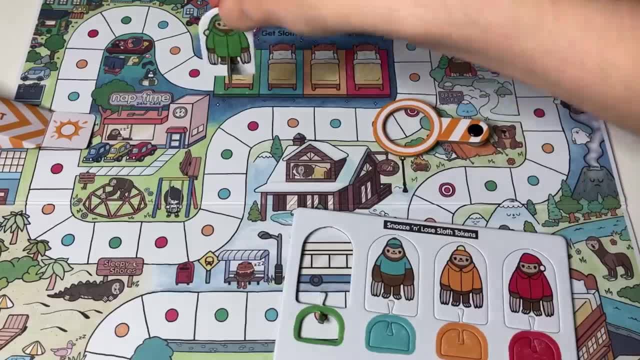 it on like that. Get my little soft guy So cute looking him, So I'm going to put him on the bed right here, And then I'm going to put him on the bed right here. So I'm going to put him on the bed. 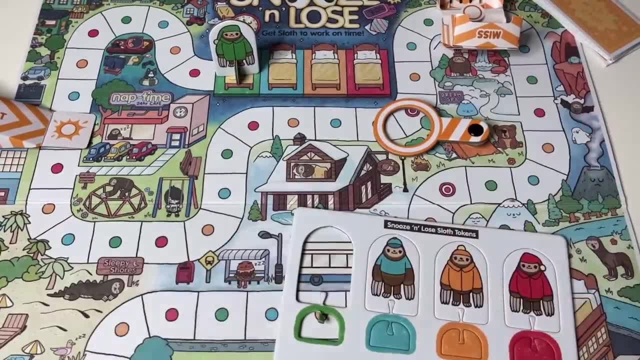 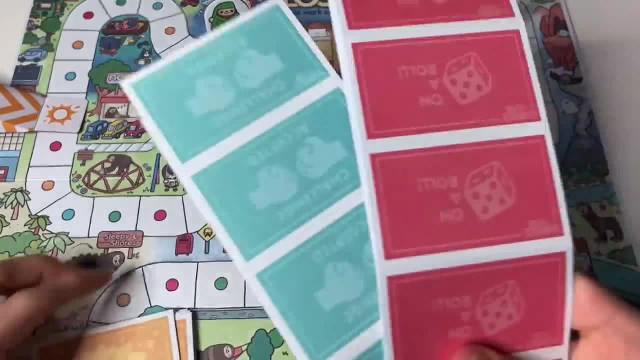 right there, All comfy and cozy, ready to go to work. So I'm going to basically set everything up right here, basically play it, And then the next day I will show you guys and review it. But first I have wild cards right here and I'm going to just unbox like, rip these up. They kind of represent. 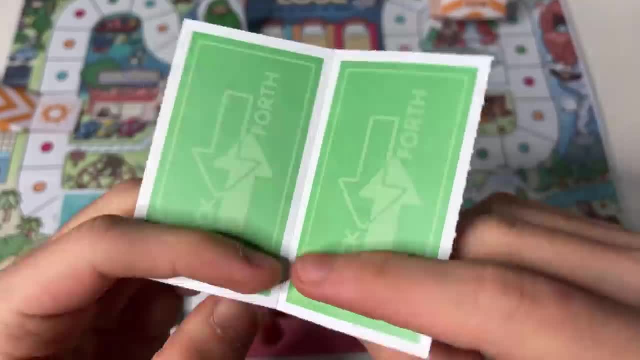 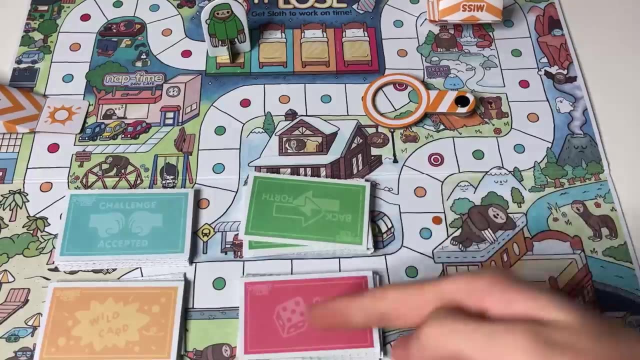 their colors. So when you land on a red piece, you get to like open the red cards and stuff, And there are a lot of them as well. So like, obviously, the more there are, the more interesting it is and it doesn't get boring. So that's really cool. So got all of it set up, I'm going to go. 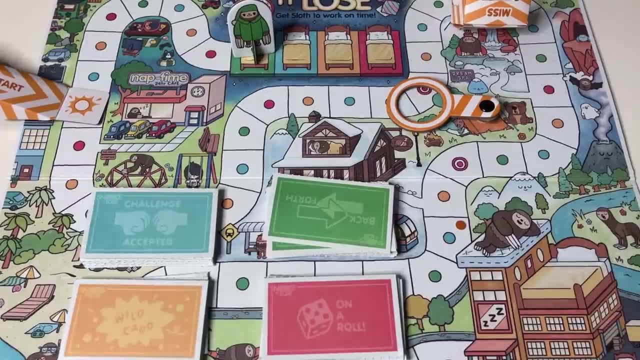 play it, Basically, review it. I'm going to go play it. I'm going to go play it. I'm going to go play it The next day, So I will see you guys in like a couple seconds for you, But for me. 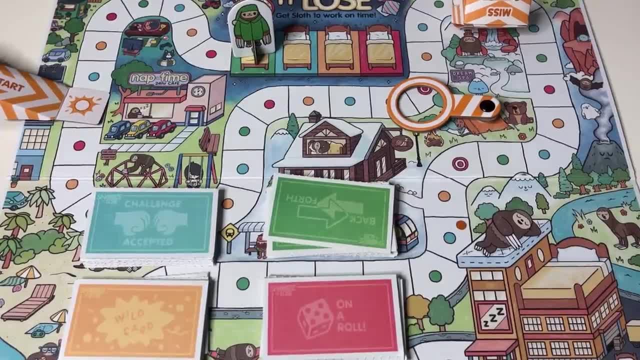 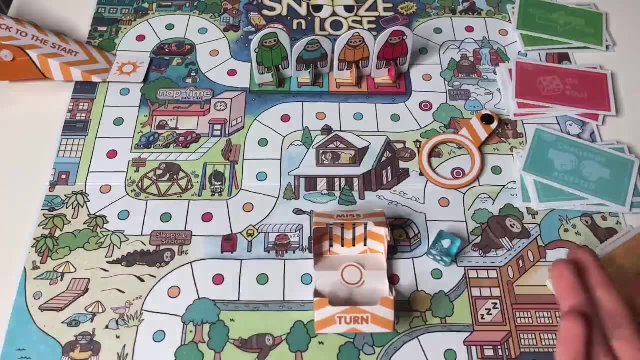 it'll be a whole day later. So, yeah, guys, see you guys in just a second. All right guys. So it is the next day and I basically played through all the whole game. I sadly didn't win, but this was so cool. Honestly, the game is so fun. Oh my gosh, It has. 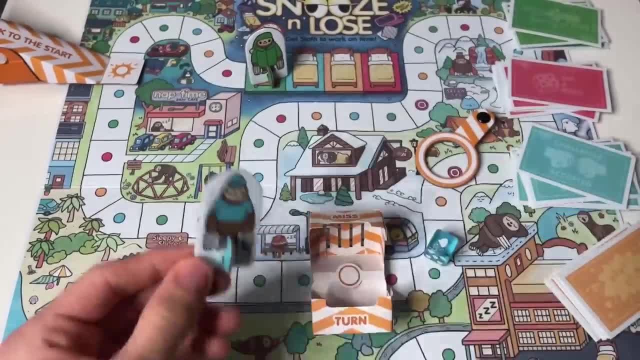 like a unique playing style and all of these are so cute. I'm going to use the blue guy because he's like the cutest and he's so small and cute. He's got a little hat on him, So I'm going to use him and basically just kind of give you like a. 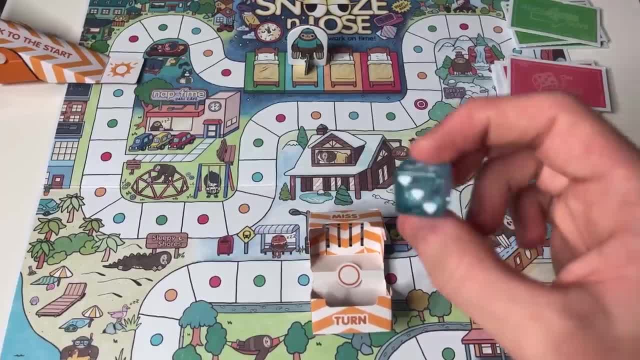 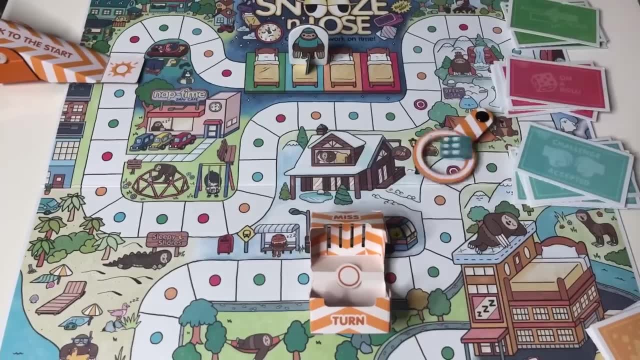 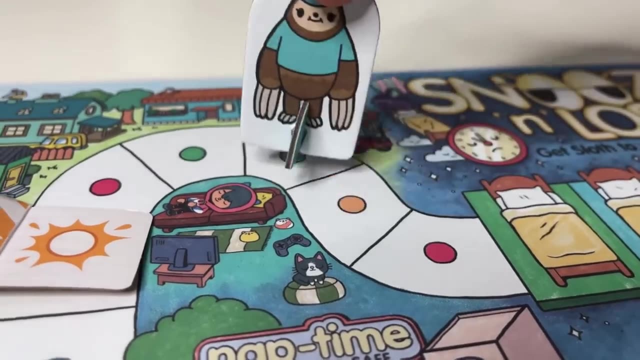 like just kind of feeling of the game. So basically, here's the dice. It's literally got poops on it, like poop little symbols, And I'm just going to roll a dice, See what I get. I get a four. OK, so that means I got to move up four spaces right here. So let's bring this guy One. 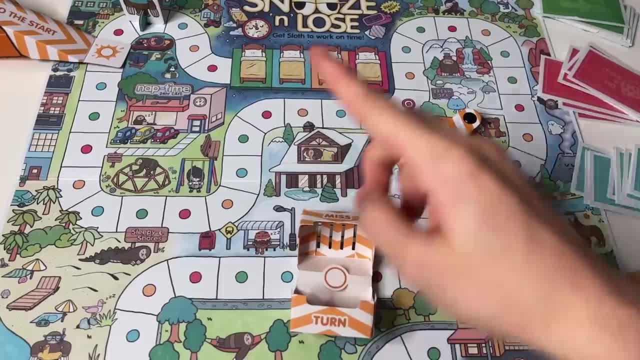 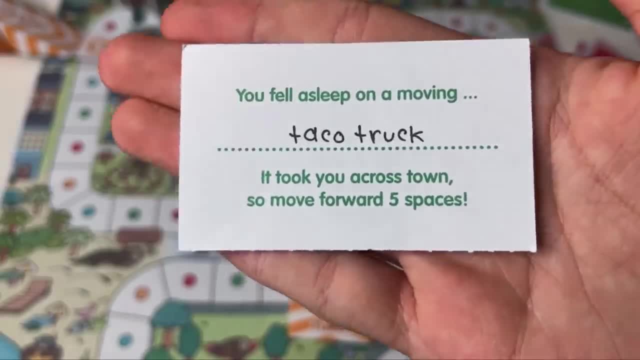 two, three, four. There we go And he's landed on the green, which means I need to pick a green card right here And it says: you fell asleep on a moving Taco truck. It took you across town, So move forward five spaces. All right, That's, that's. 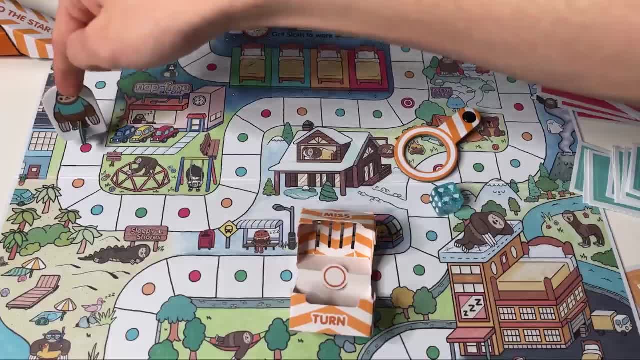 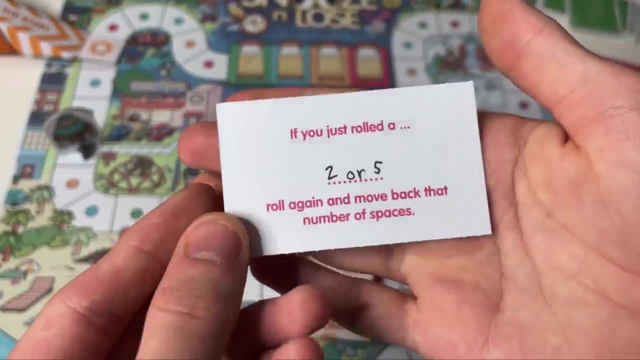 good, All right. So we're going to move one, two, three, four, five. Literally just missed the trap there, kind of, And now I landed on red. So that means, if you just rolled a two or a five, roll again and move back that number of spaces, Does that mean if I just rolled a two or five? 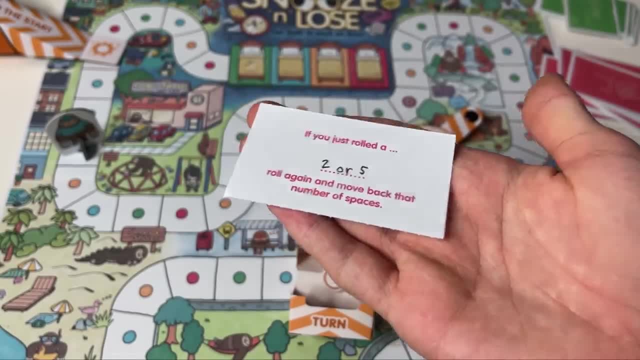 because I wrote a four, but do I have to roll it again? And if I get a two or five, I don't really. I'm just going to roll it again. If I get a two or five, I'm going to have to move back, Please. 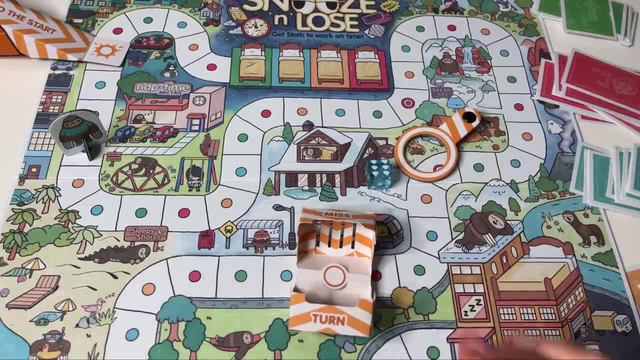 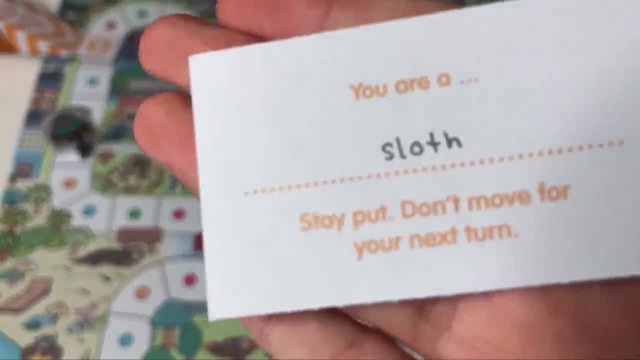 don't get to work. Okay Six, I think that's what the card meant for me to do. I don't really know. Anyway, that is honestly just so cool, Like all the traps and stuff, And these cards are like completely random sometimes, like this: You are a sloth, Stay put, Don't move for the next turn. 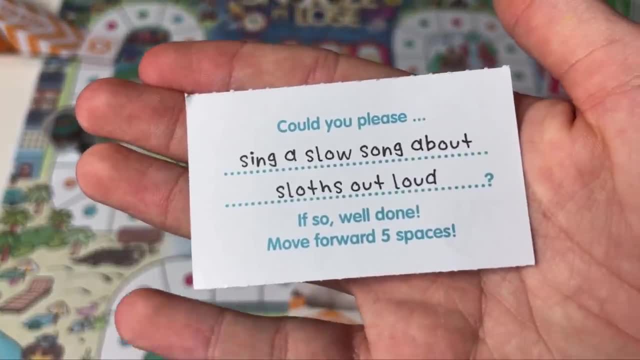 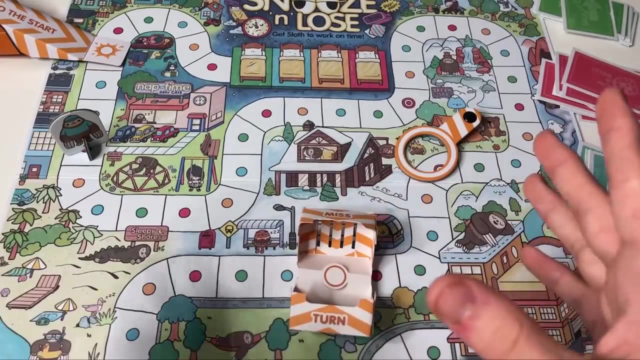 I mean, we are sloths or you get something like this: Could you please sing a slow song about sloths out loud? If so, well done. Move forward five spaces like that's. it's funny, It's silly, but it's also pretty cool And, honestly, playing this with like more people makes it so fun. 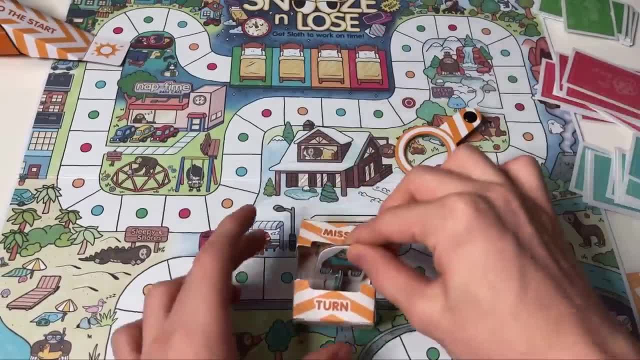 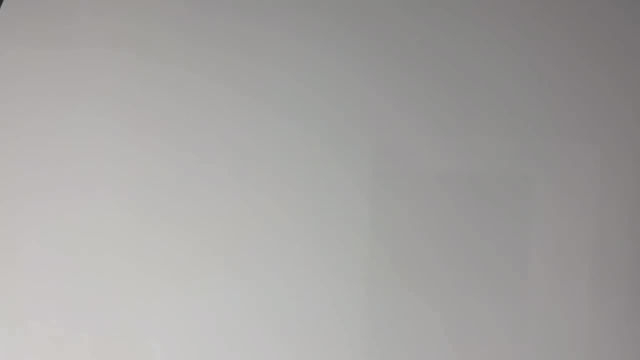 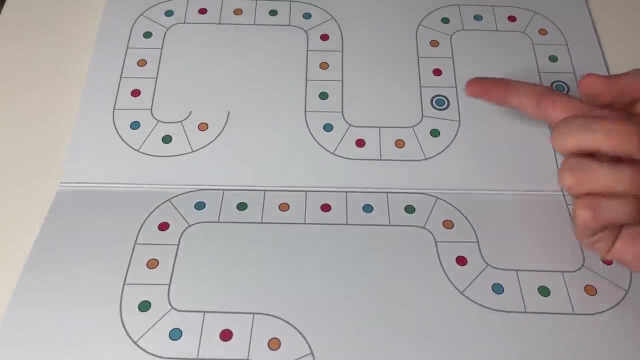 This little guy. I'm just going to go ahead and trap him in here like this: Boom, You're trapped forever. He is never getting out of there, ever. All right, Well, that's pretty much it. Now we're going to move on to creating our own board game. That is right. Let's do this. We got all the 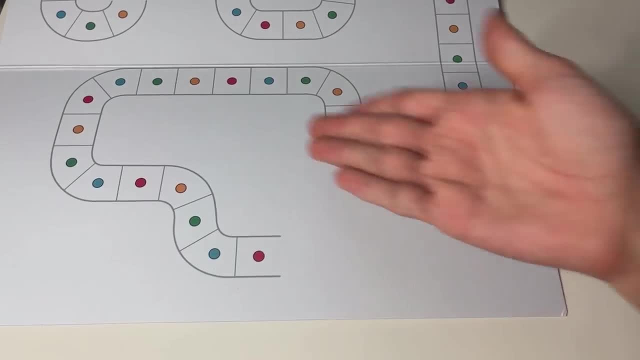 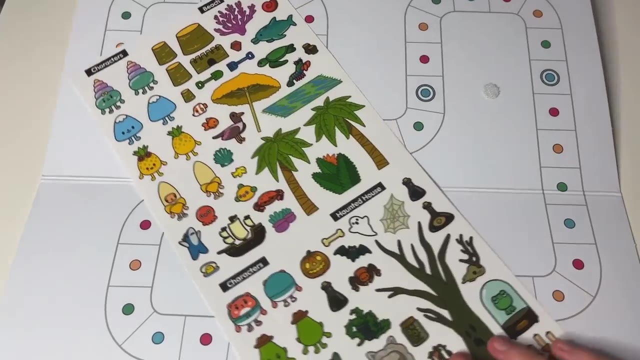 traps. We can make this to start and like this to finish, or you can make that, this finish and that to start, you know, like whatever. But today we're going to do it. So cool, I'm going to try my best. Try and do it with all of these. I'm going to try and do it with all of these. I'm going to 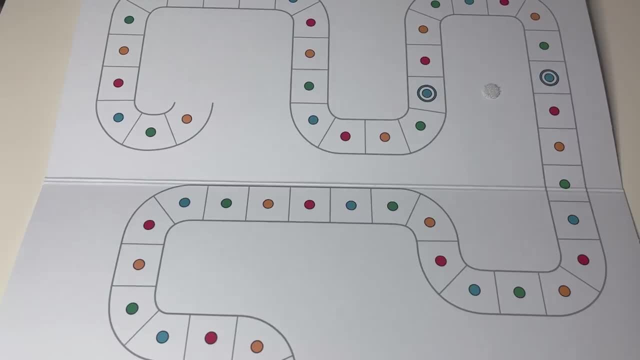 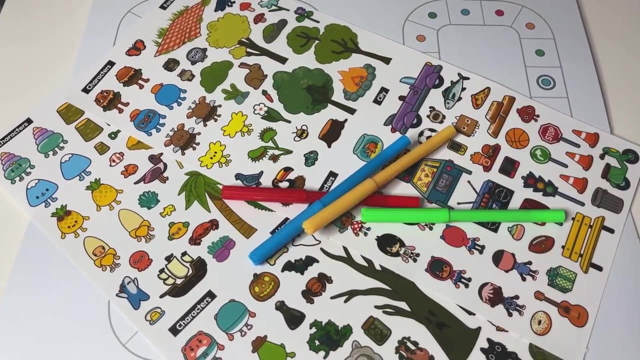 do it with all of these cool stickers right here and, you know, customize it, draw on it with the all these stickers. There's so many, There's so many. So yeah, And I've also got all these kind of pens right here and we're going to do it. So, first of all, this is me drawing this thing, right. 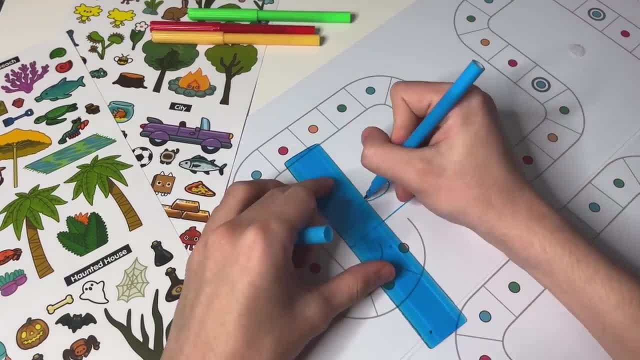 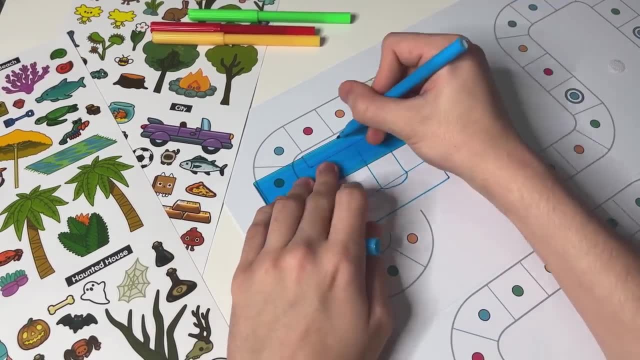 here. So this is the start. Now I'm drawing something. Can you guess what it is? So I'm kind of going for like a city kind of parky vibe, So like the style of it. So it's going to be like: 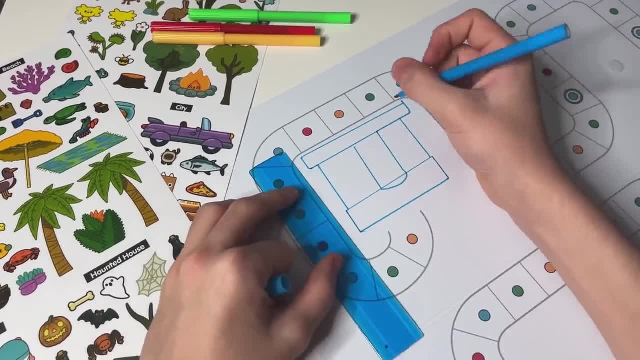 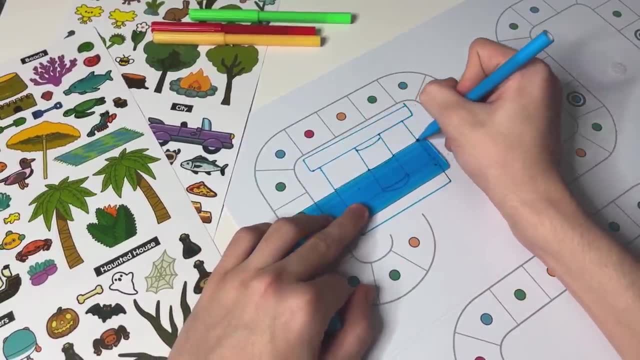 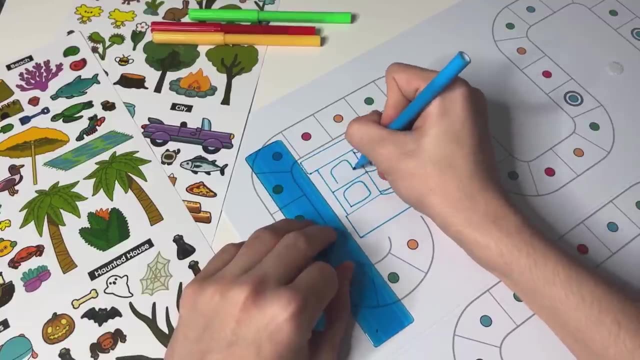 just basically mainly city and like forest. But first I'm drawing a building very recognizable in Toka Life world And it is, I don't know, Can you guess it? Maybe Yes, No, All right, So it is the apartment place And I'm just drawing all. 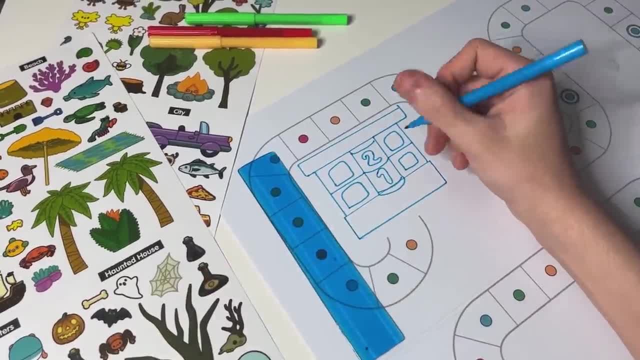 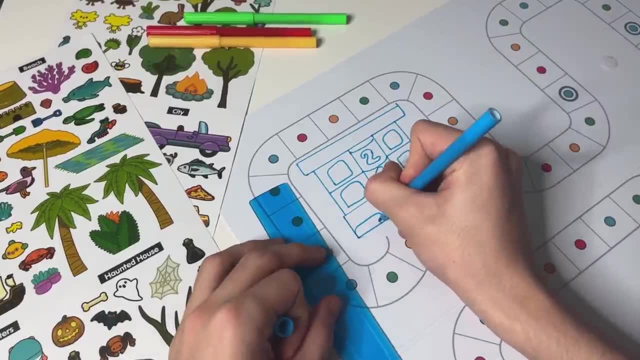 the windows, And basically every window is a starting point for the four players, So they start there. on the windows, We got the little door there. I'm honestly not the best drawer in the world, So I'm just kind of like, you know, just trying my best, But I have a little ladder right. 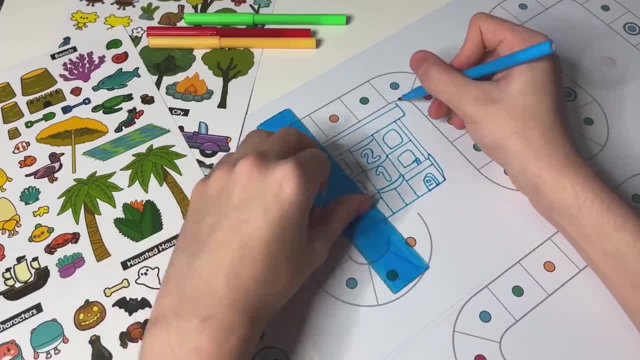 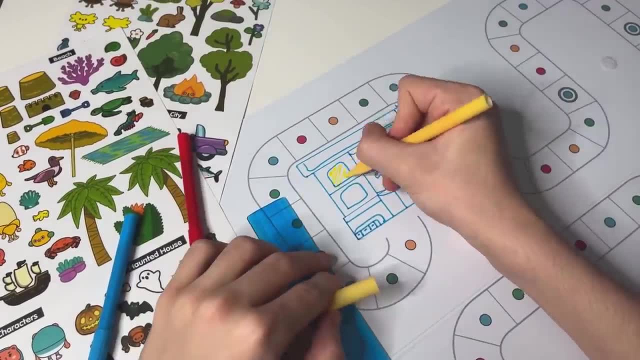 here And I'm just kind of trying to make it 3D And you know I'm just I'm really not that good of a drawer, But you know I try my best And I just add a bit of color as well, You know. 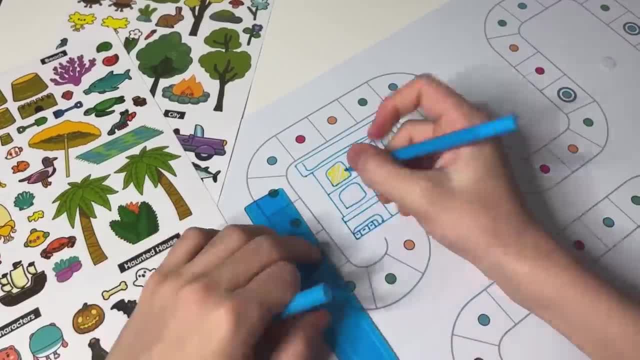 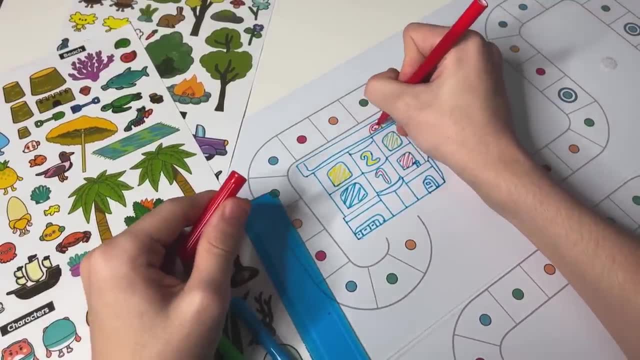 highlighting stuff. Every window is represented a different color for every player, And I just add a cute little sloth on the top here as well, Because why not? Who loves? We all love a good sloth, right. Look how cute that guy is. He's so cute. Look at him. He's chilling up there. 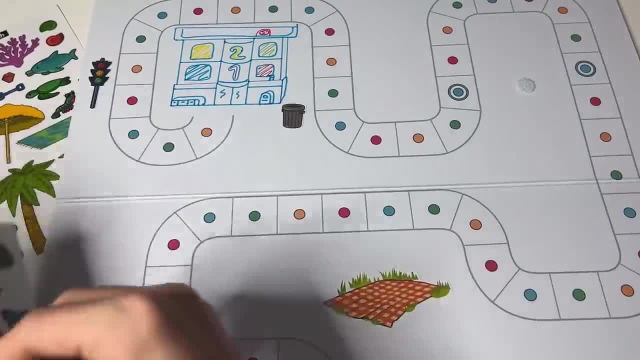 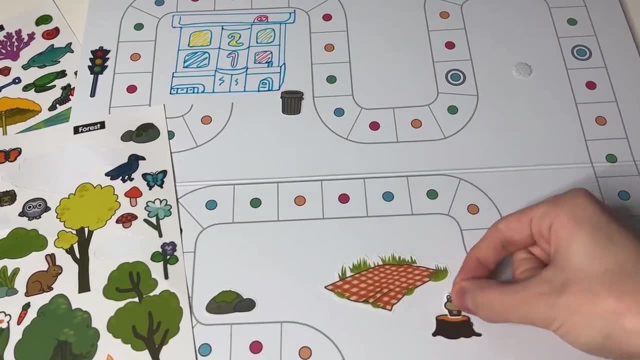 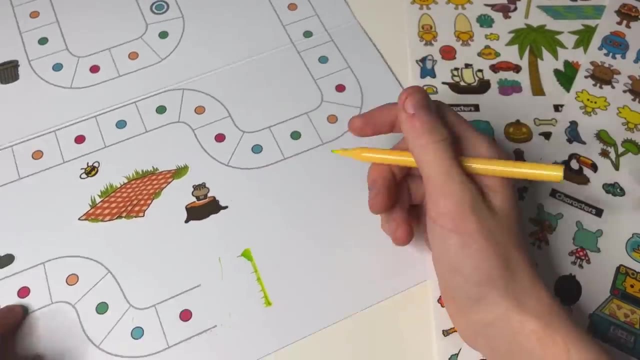 But anyway, add a few stickers. I add this kind of you know parky design. So I add like a stump and a picnic blanket and stuff like that, A little squirrel just down here at the bottom, Little bumblebee flying, And then over here, as you can see, my yellow pen kind of smudged a bit. 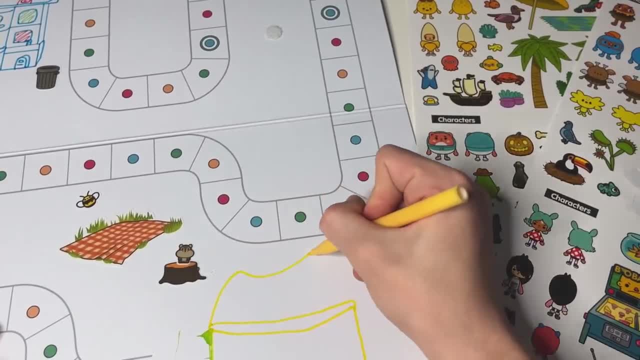 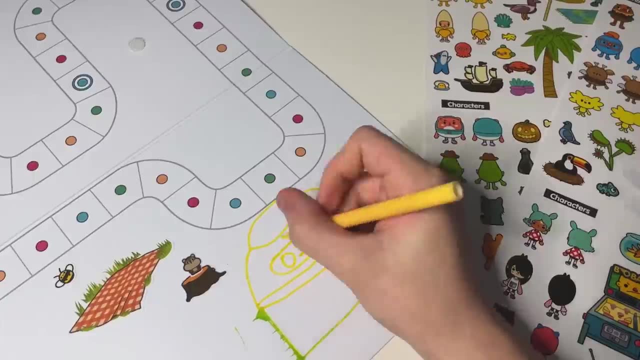 I'm not going to use the blue ruler because it kind of smudged my yellow pen, which was so annoying. But can you guess what I'm building, Building What Drawing This time? you can probably tell from the face already. That's right, RoboCafe. 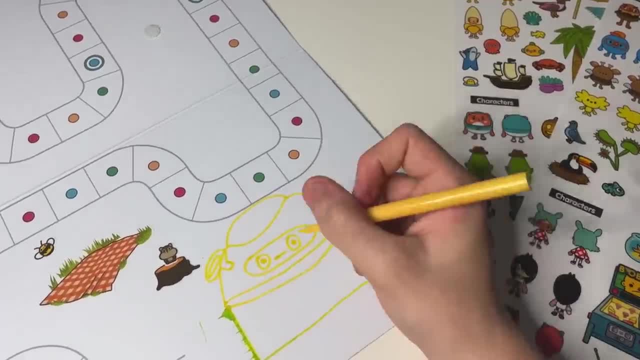 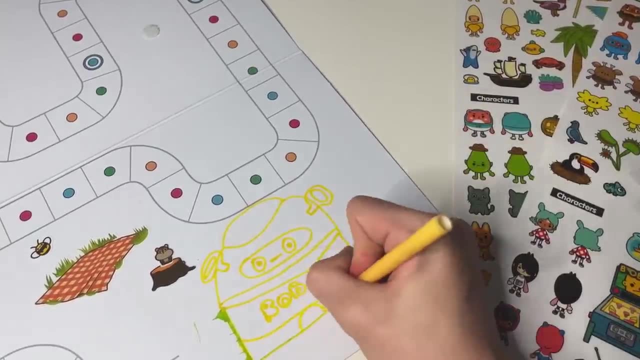 They have to finish at RoboCafe. So basically I'm going to have the characters as the gang. They start at the apartments and they basically go all the way over to RoboCafe And that is where they finish off, like that, Perfect. So I add a few designs And again, as you can tell, 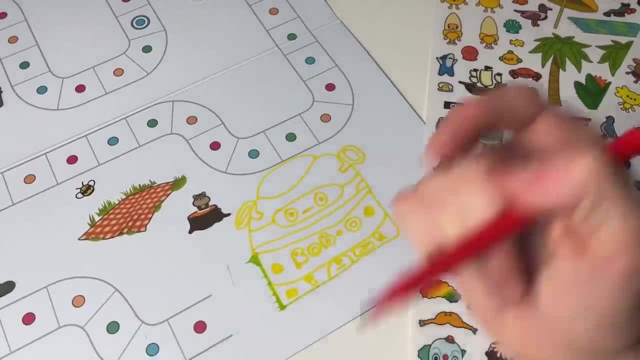 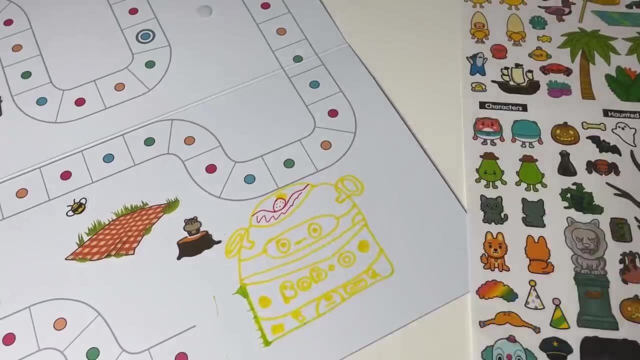 I'm really not a good drawer, but I'm trying my best And I just add like some nice little strawberry mix at the top here, like in the game, And that is just kind of mixing around up there a bit. There's my little RoboCafe, Very derpy, But I also add a few. 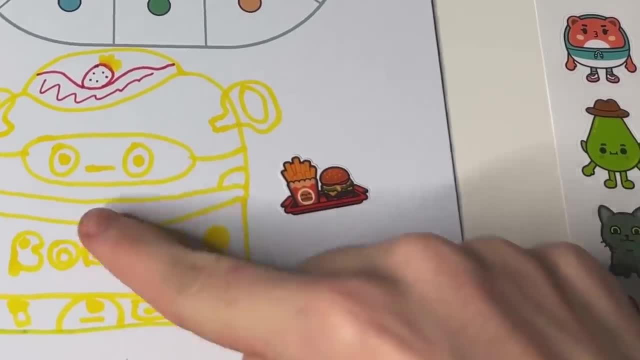 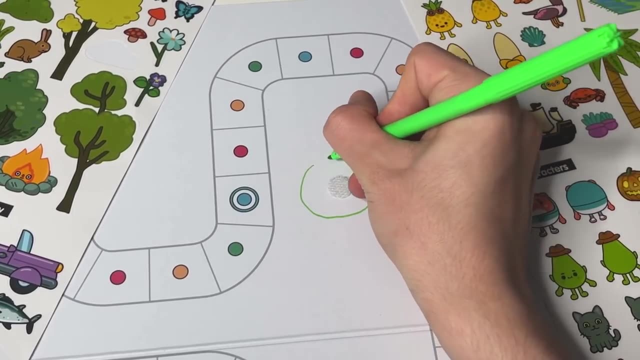 stickers. I had a bit of goodies behind it like food and gold and stuff, because once you enter RoboCafe you're behind RoboCafe and get all of these cool goodies. Now, on this Velcro thing, I'm drawing Floople, which is on the character creator thing with a huge nose. So I made the 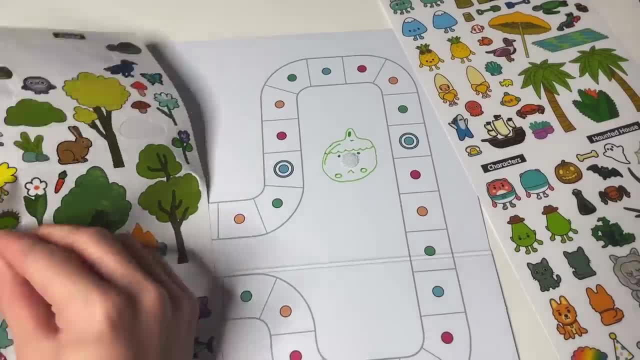 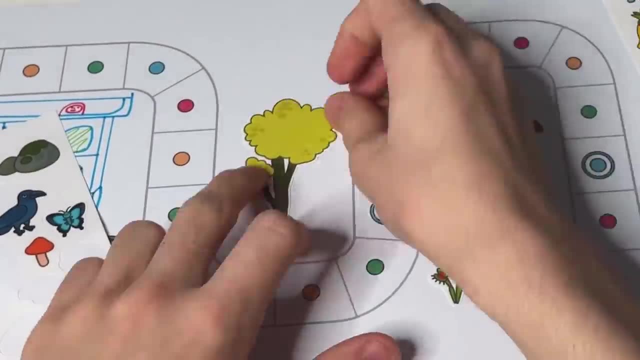 Velcro like a huge nose, I don't know. I just thought it'd be funny to do that And I add a little like greenery stuff around him Like this: just a few flowers and stuff plants a big tree in the middle right there, which is nice. 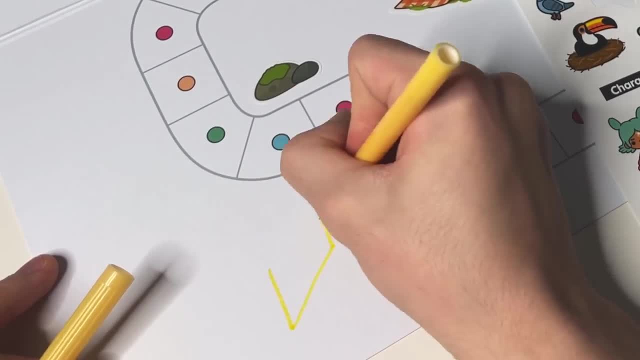 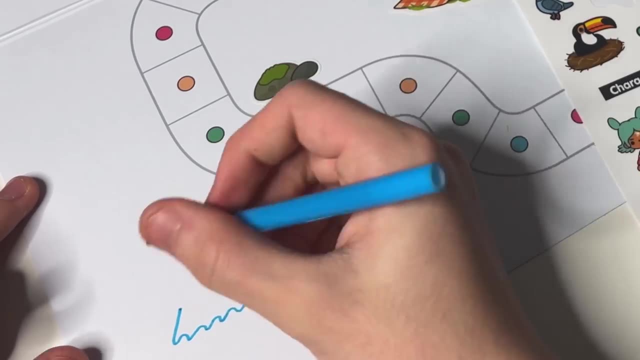 And then I also start to draw something which maybe you guys could guess what it is again. So you're probably going to guess eventually. but here's a wall, And then we have a blue roof right there Just drawing that on, And then I'm add a little bit of here And then I start drawing. 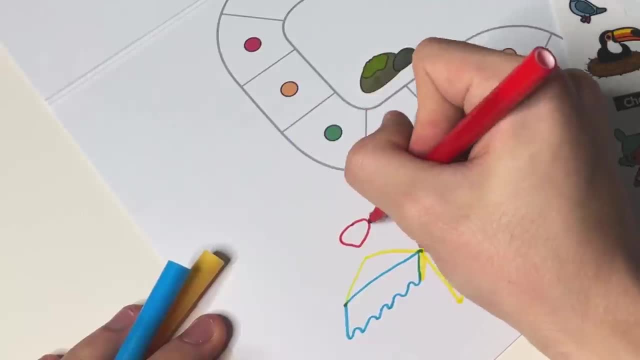 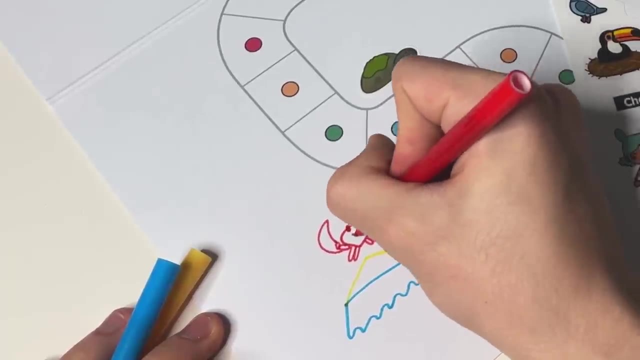 in red. You probably tell from this bit Again, I'm not a good drawer, but here we go, Add this claw right here. Yes, that's right, I am drawing the krill krill. So this is going to be this kind of like a little. 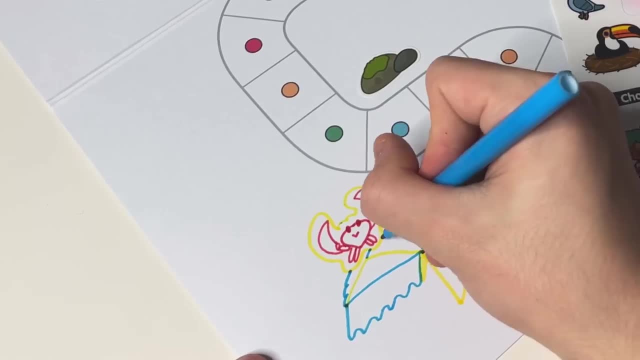 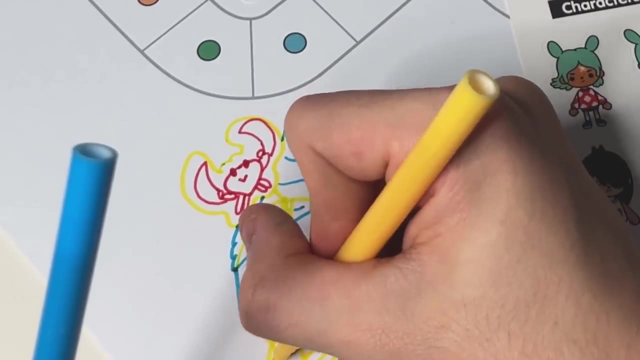 background bit right here. I'm just going to add another blue roof there And I was just trying to copy off best what it looked like in the game. But I just add the little balcony bit over here with the doors and stuff because it's like the nice little patio And honestly I love this location. 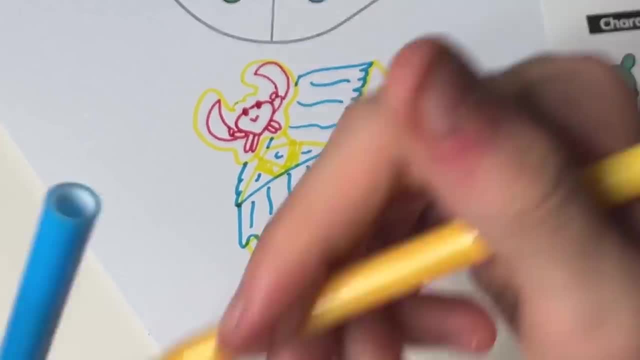 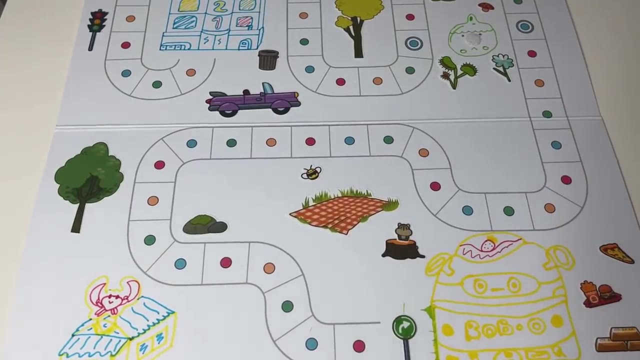 in the game. It is literally so good. I honestly love it. I love all the new foods they added as well, like the calamari and stuff. There's my krill, krill all done And I'm just adding a few more stickers to kind of brighten up the place, make it a little bit more. 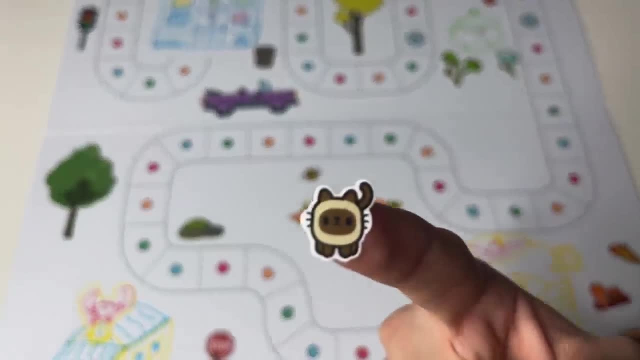 better And I found this guy. That's right, It's Cookie from my Toka Life series. If you haven't seen it, this is Cookie the cat. He's so cute And he's a sticker, So I'm going to place him. 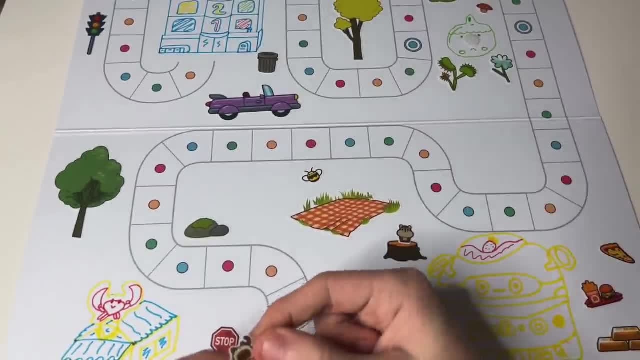 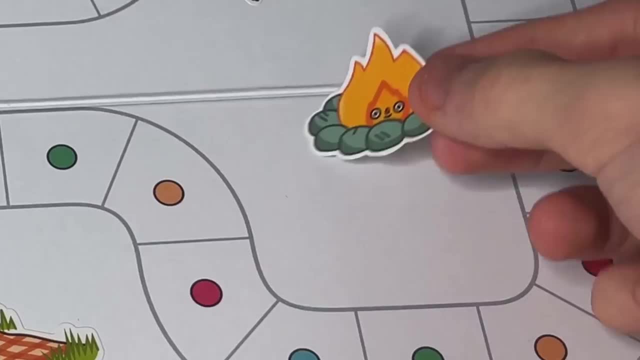 on the what's it called The picnic blanket. So yeah, I'm just going to put him right there. He's going to chill, So cute little cookie. Look at him just chilling there. All right, So I'm just adding a campfire right here. Just right there. Stick it right there. Just a little cozy bit. 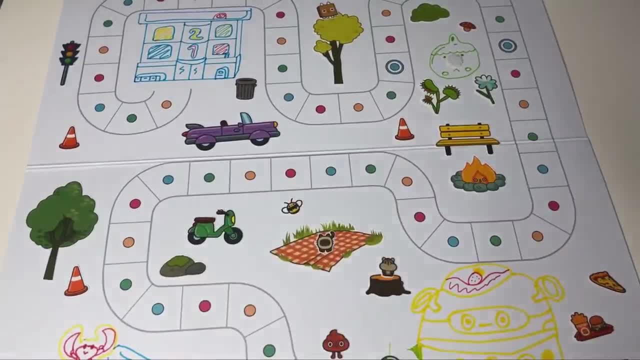 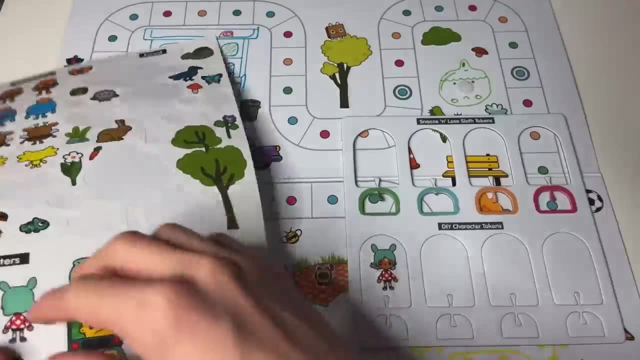 A few more stickers just to make it a little bit more better. And once my stickers are all placed down, I start adding the characters in right here. So I add Rita, of course, and add behind here as well, So you can see the back, which is very cool, Actually I like that. And then I just add: 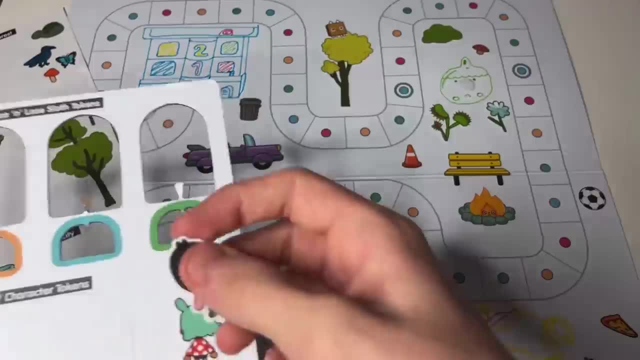 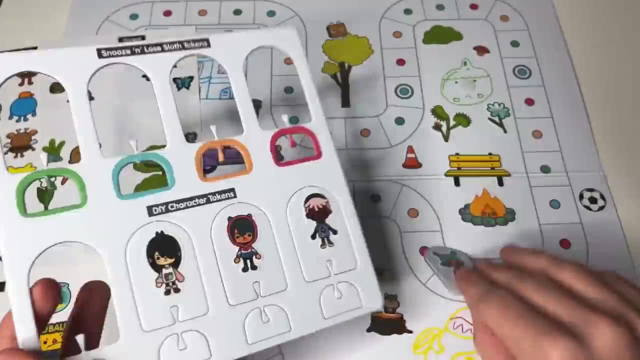 Nori as well and put hair on And I also add Zeke and Leon and stuff like that. You know the whole gang, because they're ready to hear and they're ready to play. So I'm just going to pop them all out right there, like that. 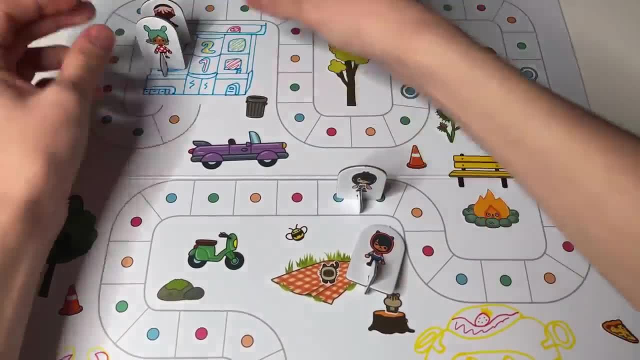 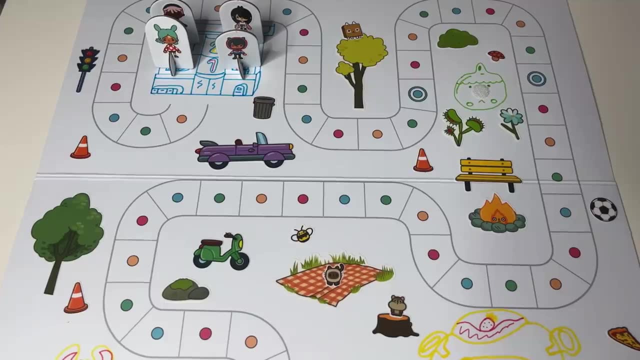 And then, once I've got them all done, I'm just going to place them on all of the four windows ready to start the game. Let's do this. There we go. Perfect, All right, Okay, This is so fun. I. 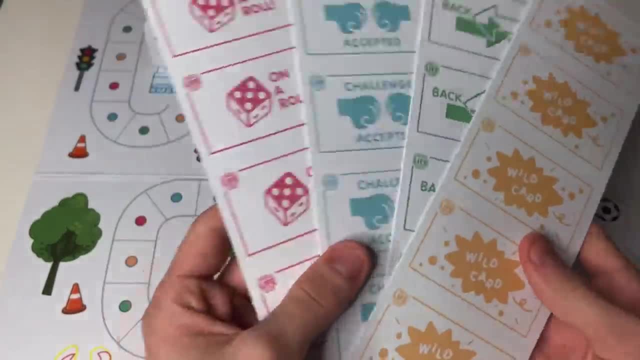 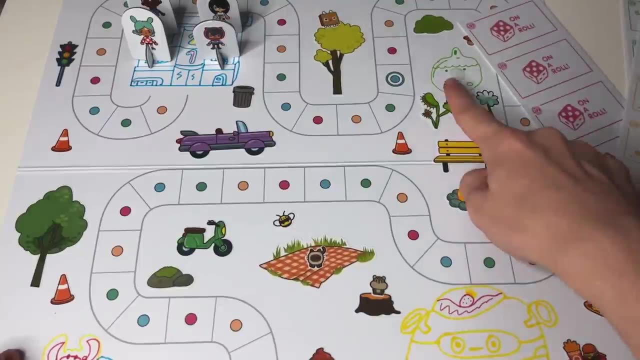 love creating my own board game. This is- I never thought it'd be like this- fun. But then I also have all the wild cards which I'm going to like draw myself as well, Kind of come up with some cool ideas. But this flute ball is so cute And I need to add the trap on him as well. But honestly, 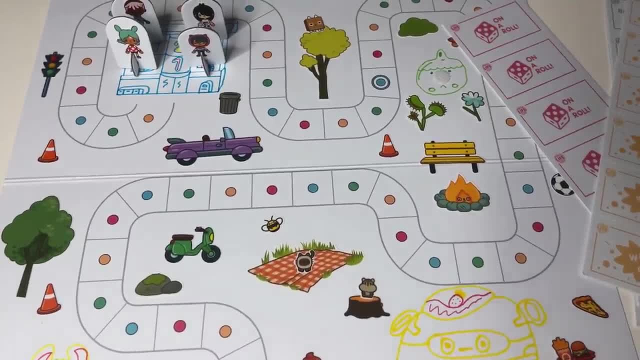 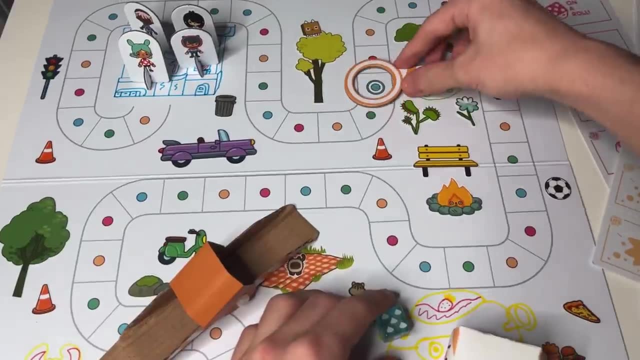 creating your own board game- literally so fun. You can come up with anything you want. Like, you don't have to do this. You could just go for, like the haunted house vibe or something as well, But I'm just going to add the trap right there. The Velcro bit just kind of turns around from.